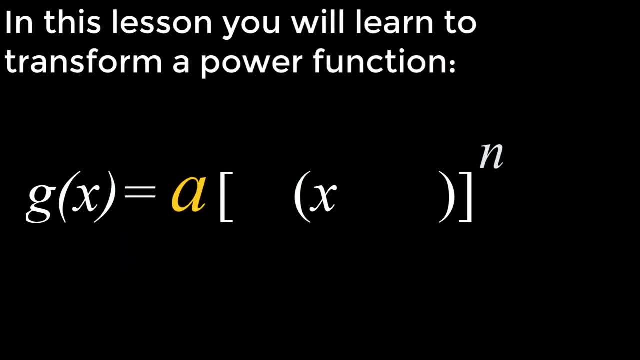 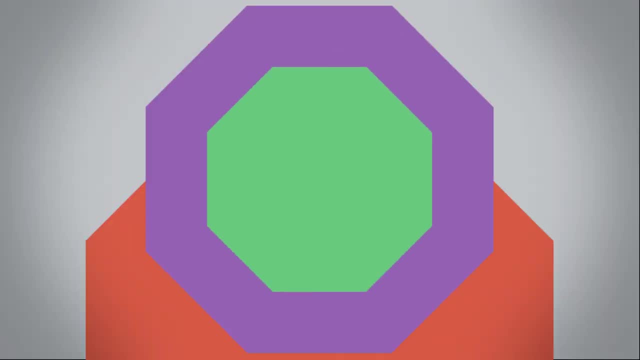 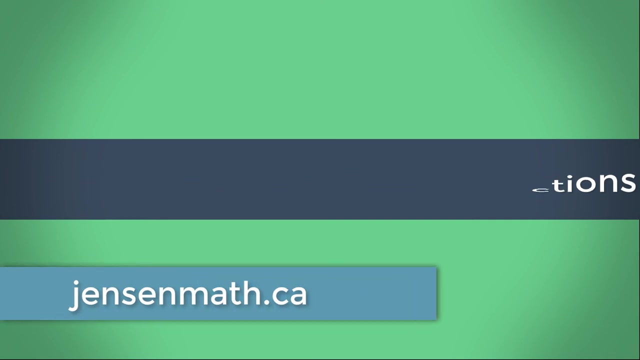 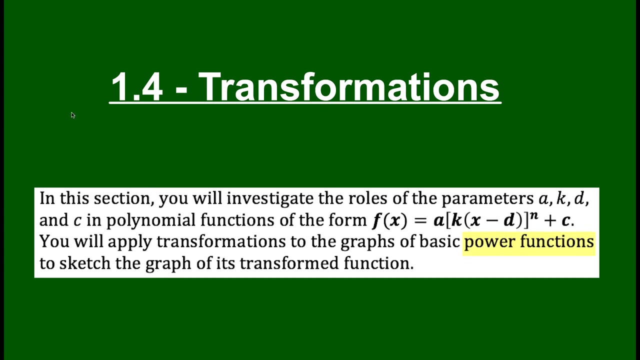 This is lesson four on transformations. So in this lesson we're going to be doing transformations of power functions And we learned what power functions were earlier in the unit So you should remember from previous courses what the parameters a, k, d and c do to transform any function. We're just going to apply those. 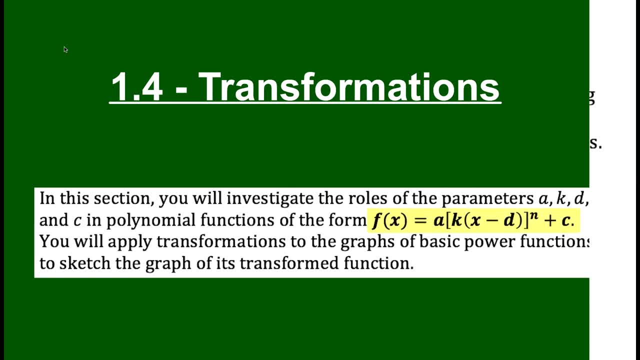 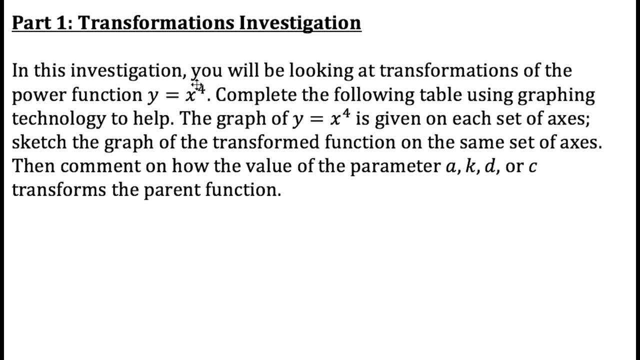 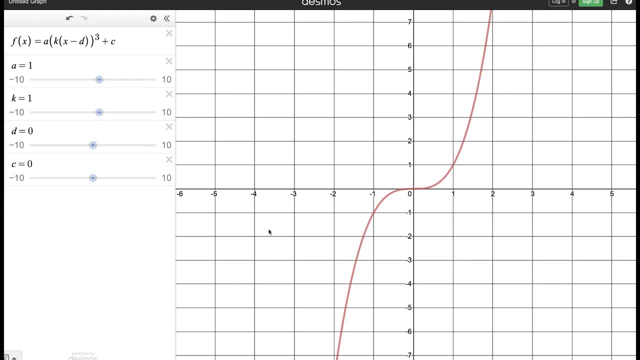 parameters to power functions. like you see here, Before I take you through the investigation where we do transformations to this power function, x to the four, let me just open up Desmos and give you a quick visualization of what those parameters- a, k, d and c- do to transform a function. So here, 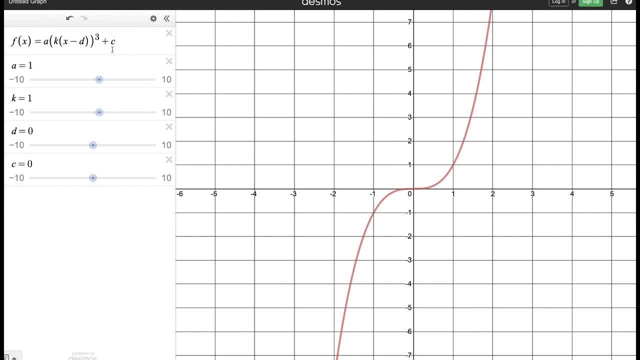 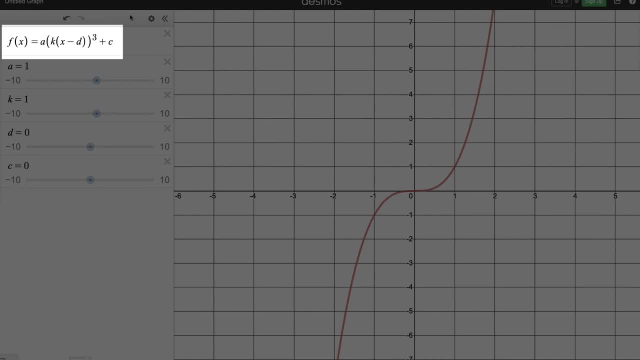 in Desmos I have this x cubed function And to that x cubed function. right, we can see this is an x cubed function. I'm applying the transformation parameters a, k, d and c to that x cubed function. 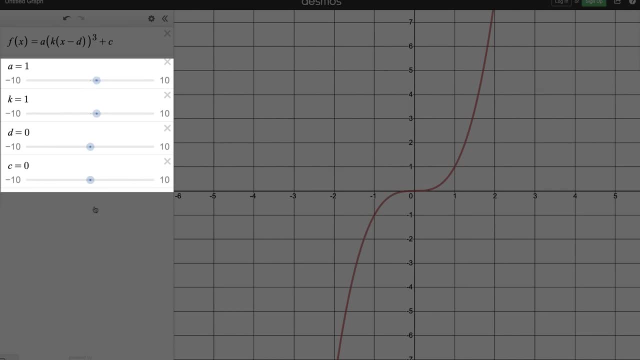 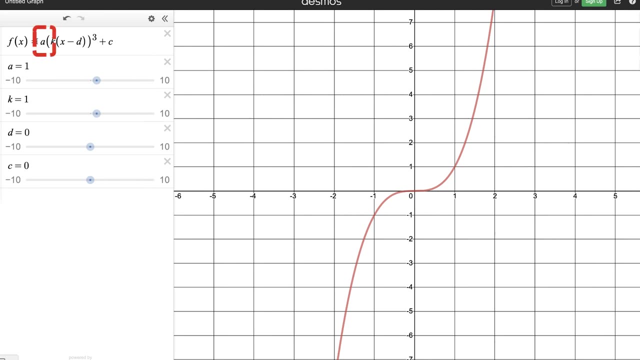 Let's just quickly play around with those parameters to get a refresher on how that affects the shape of the graph. The first thing I want you to look at is the parameter a. Now the a parameter, which is the factor in front of the power function, can do a couple different things. 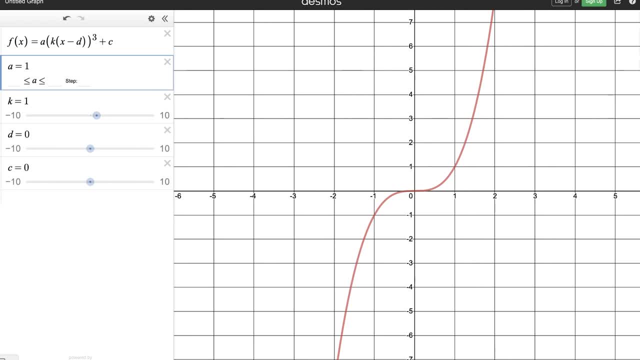 If I make a negative, it's going to do a vertical reflection. Hopefully you can see that vertical reflection happening as I made it negative. But it can also do a vertical stretch or compression. So watch as I manipulate this a value. It could do a vertical stretch if the a value is bigger. 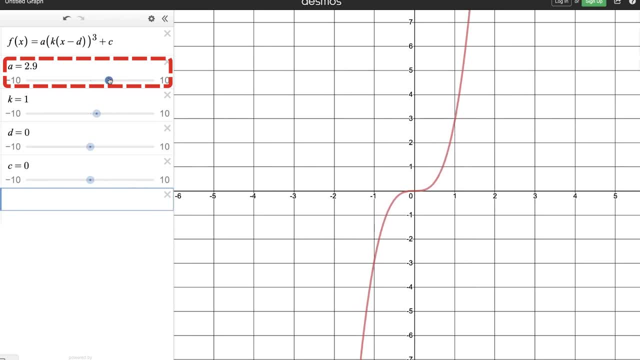 than one. So imagine someone grabbing the ends of this and stretching it vertically. It would also do a vertical stretch if the a value is less than negative one, So let me set it to negative one. So now it's going from quadrant two to four instead of three to one, because it's 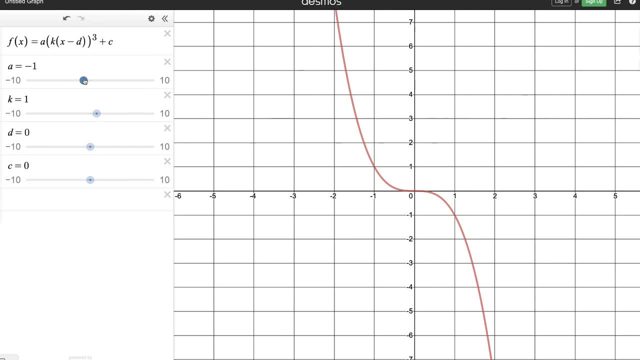 been vertically reflected, and now let me make this a value less than negative one and notice it's also getting vertically stretched. If I let a equal something between negative one and one, it's actually going to do a vertical compression Picture. someone squishing it from. 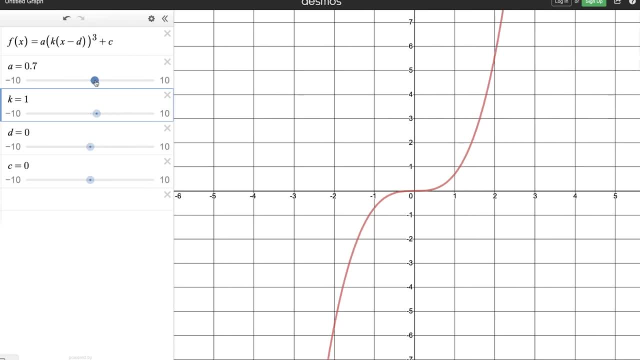 above and below and you'll see what's happening. So the parameter a actually does a vertical stretch or compression by a factor of the absolute value of a. if a is negative, that just causes the vertical reflection. now let's look at the k parameter and what that's going to do to transform a function, and that's actually going. 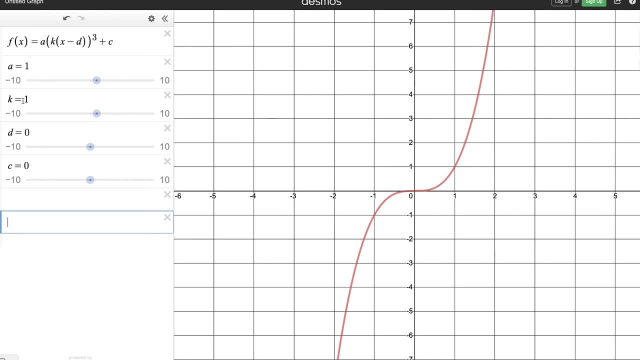 to do horizontal stretches or compressions, and it could also do a horizontal reflection. if k was negative, watch as i make k negative, picture it flipping horizontally across that y-axis. now for an x cubed function, you might say, okay, well, the horizontal and vertical reflections actually do the same thing, and you're right. for for an odd degree power function, that'll be the. 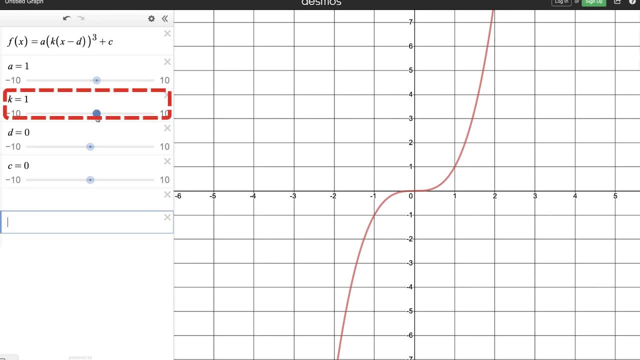 case. but let's watch what happens as i make k bigger than one, it's actually going to do a horizontal compression by a factor of one over the absolute value of k, and if i make k less than negative one, let me set it to negative one. if i make it less than negative one, once again horizontal. 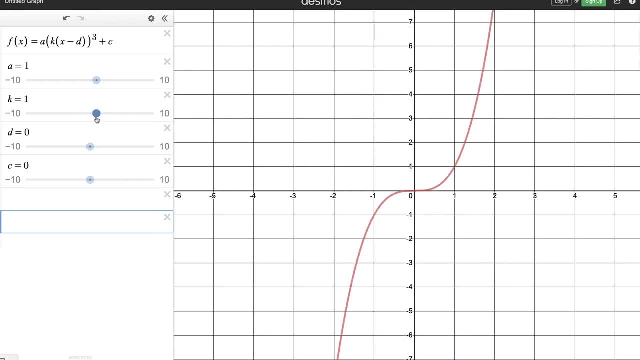 compression by a factor of one over the absolute value of k. if k is something between negative one and one, it does a horizontal stretch by a factor of one over the absolute value of k. picture someone grabbing the sides of this and stretching it out: you the d value. if d is something bigger than zero, like, let's say, three, it's going to shift right. 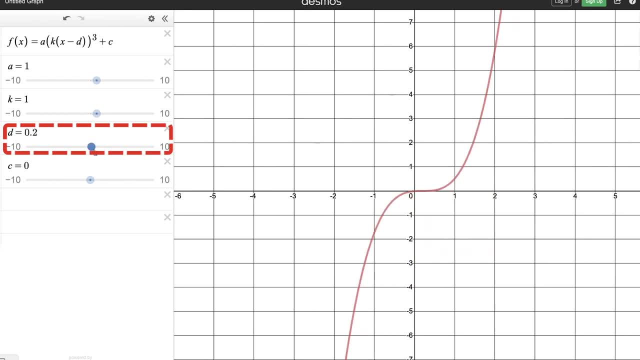 three. if d is something less than zero, it's going to shift left by the absolute value of that amount. so if i make d negative three, notice it shift left three. now if this d value of negative three was in this equation, it would be x minus negative three, so it would look like x plus three. but you would 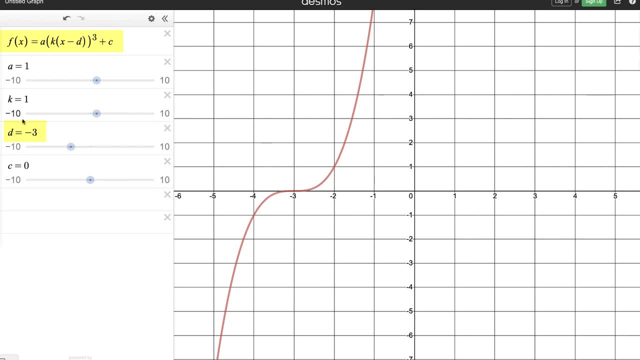 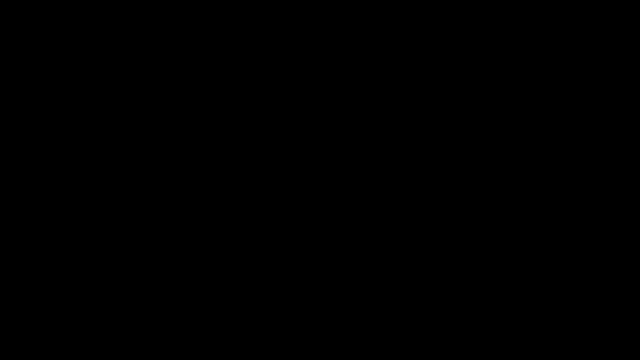 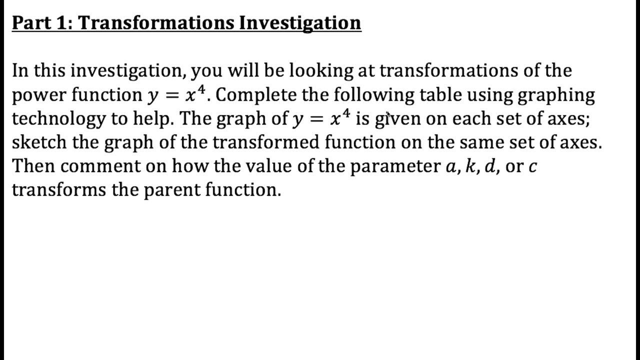 have to know that, based on this format of the transformed equation, the d value would actually be negative three, and a c value shifts it up and down. okay, let's complete part one of this lesson where we're going to kind of go through an investigation like a. 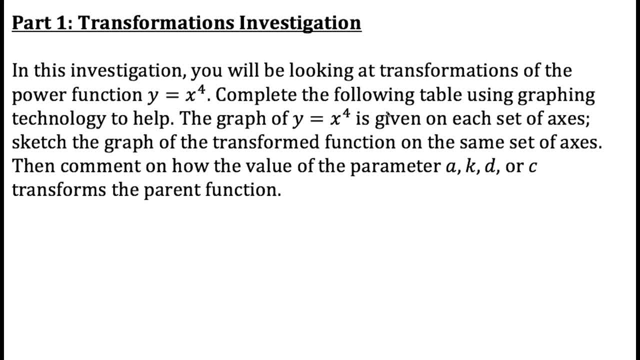 test that is showed you in desmos, but we'll actually record our answers. so in this investigation we'll be looking at transformations of the power function- y equals x to the four, and we'll complete a bunch of tables of different transformations. so we're going to go through the 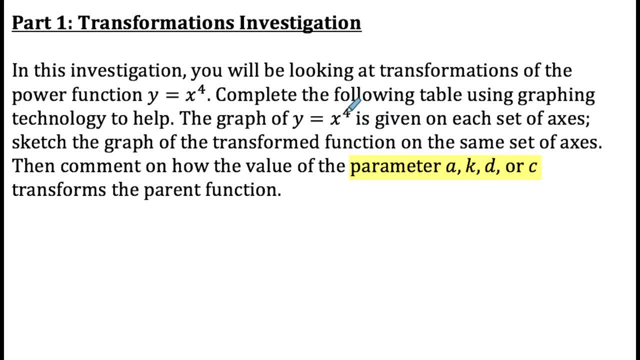 parameters a, k, d and c, one at a time, to show how they transform the function. y equals x to the fourth. it's important to know that the parameters k and d are going to affect the base of the power. they're the horizontal transformations, so the base of the power would become k. 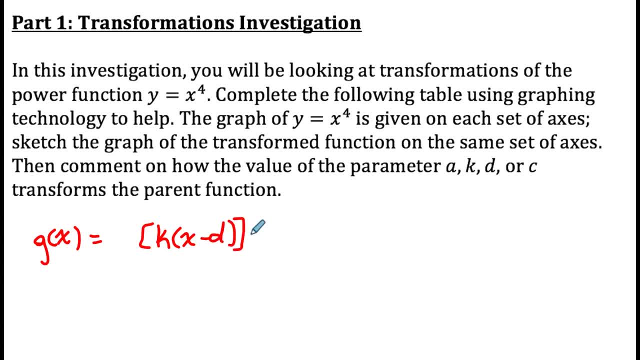 times x minus d, and the exponent of four will be on it, because this is a transformed x. to the four function and then to that power, the vertical transformations happen. we multiply it by a and we add c. so notice the location of the parameters a, k, d and c and let's go through. 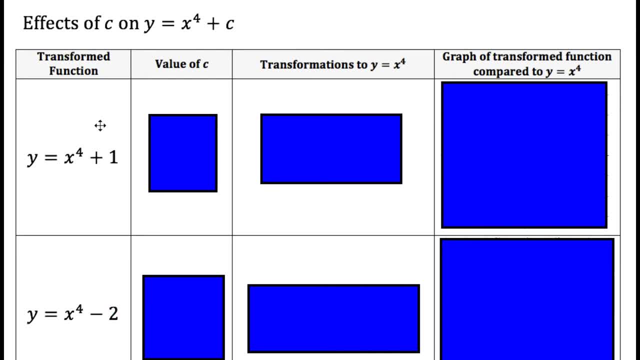 what they do one at a time. so let's start by looking at the effects of the parameters c on the x to the four power function. so if we add c to the x to the four power function, what happens? so in desmos i've changed it so i now have the x to the four as the parent. 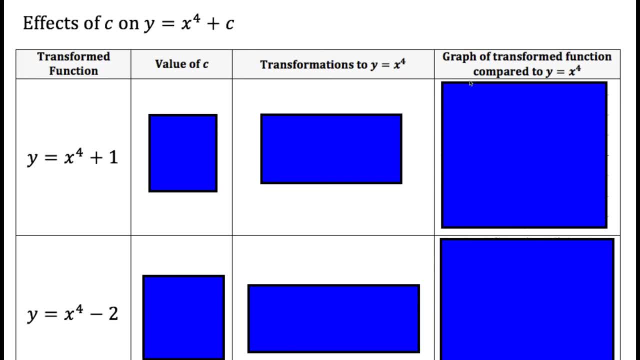 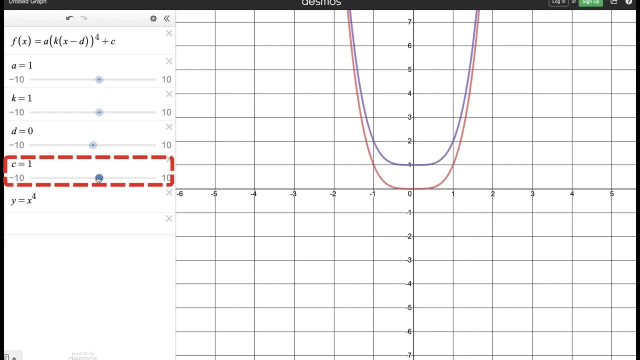 function and we're going to apply transformations to it. let's manipulate c first. so in this one's the c value is one. so if i make the c value one, let's look at what happens. notice the transformed function. the purple one is one higher than the parent function. x to the fourth, so it's been. 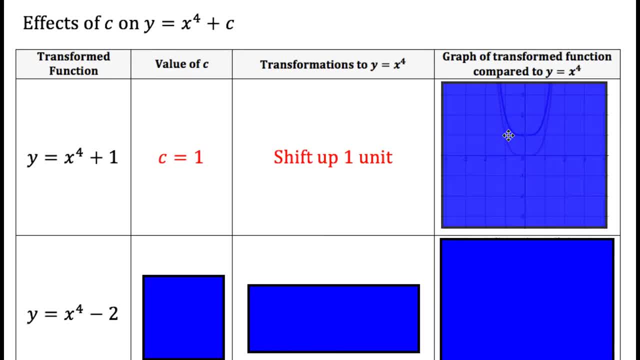 shifted up one and just do a quick sketch of the graph. that is one higher than the parent function. you're given this red graph, just sketch the purple. one should look exactly the same, just one higher. and then let's make the c value negative two and see what happens. so if i change the c value to 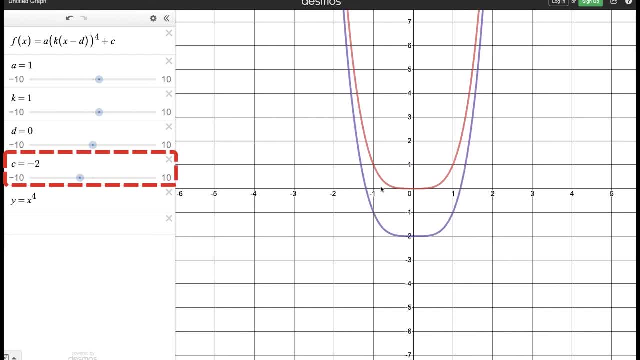 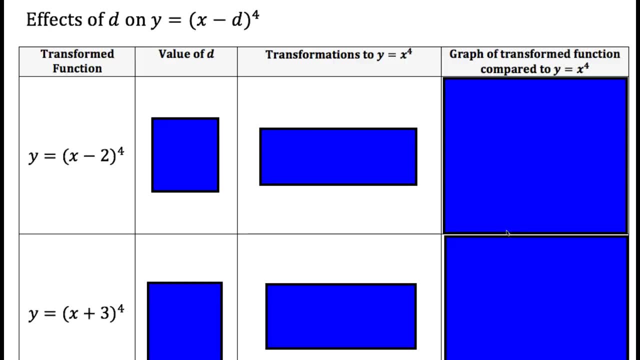 negative two. notice the transformed function is now two below the parent function. exact same shape, just been shifted down two units. you can sketch that graph as well. let's look at the effects of the d value. remember the general format is x minus d. so in this equation, x minus 2 to the power of 4. 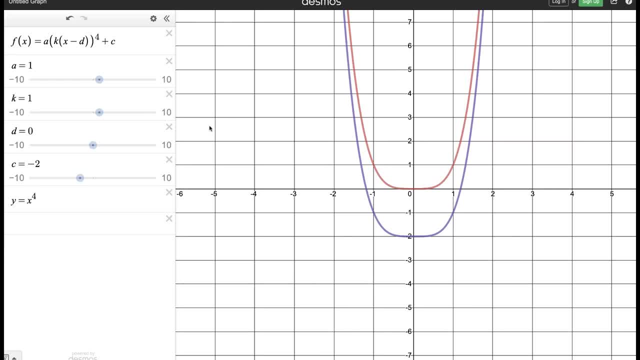 the d value is as follows: 2. Which let's look what happens if the d-value is 2. So let's set the d-parameter to 2, and notice that it shifts it right two units. So it shifts it right two. 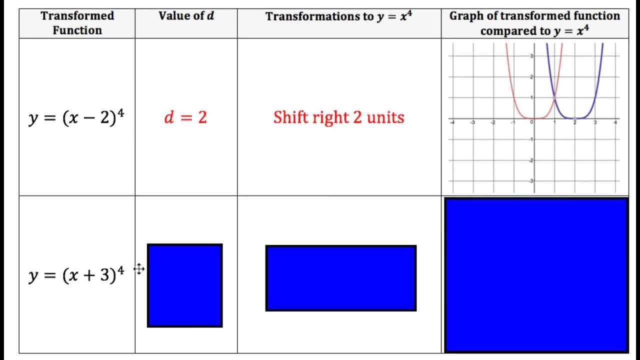 units. you can sketch that graph For this transformed function. it looks like it's an x plus 3 to the power of 4.. In order for it to look like this, the d-value must have been negative 3, because if I plug negative 3 into this equation up. 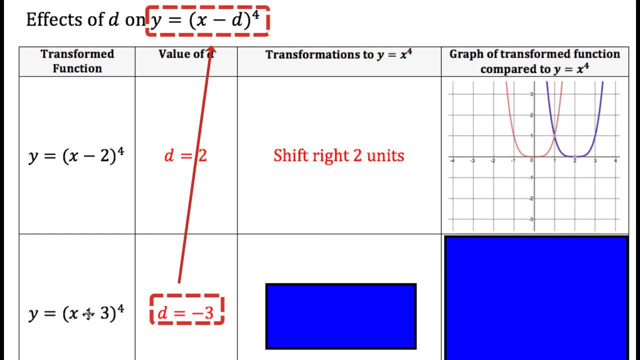 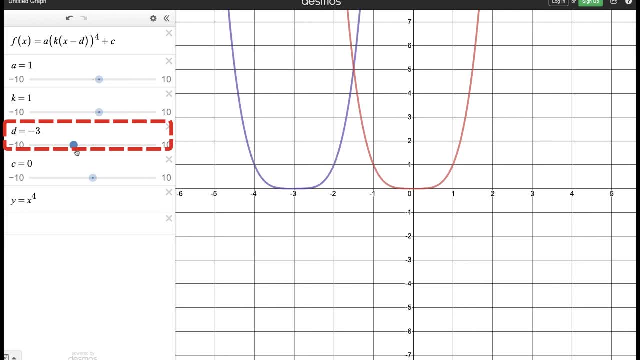 here it would be x minus negative 3, which simplifies to x plus 3.. So what does a d-value of negative 3 do? Let's make the d-value negative 3.. Notice, compared to the parent function, it has been shifted left 3.. So you can sketch. 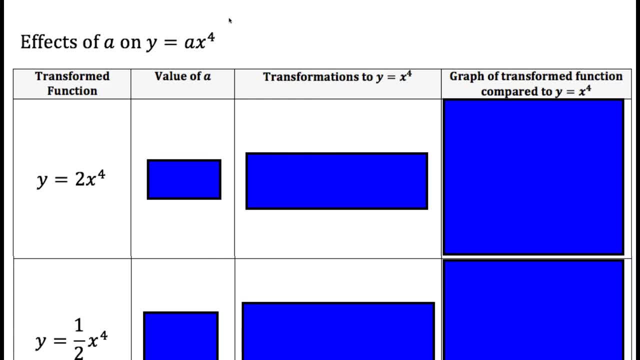 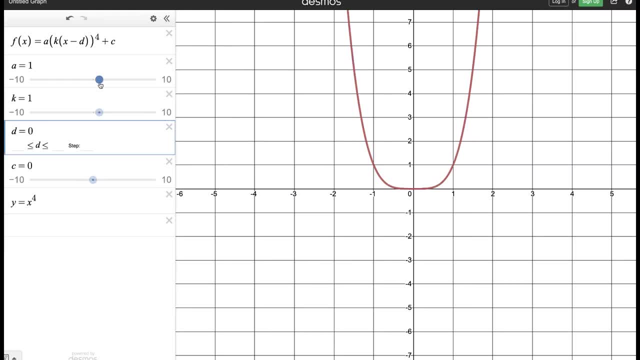 that graph as well. Now let's look at the a-value. So the a-value is the factor that's in front of the power. If I make the a-value 2, let's see how that affects the graph of the parent function. Notice: 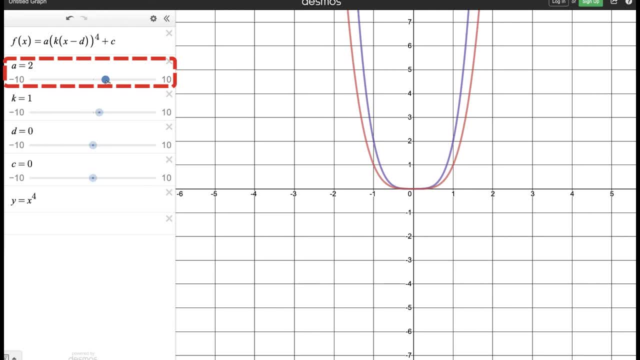 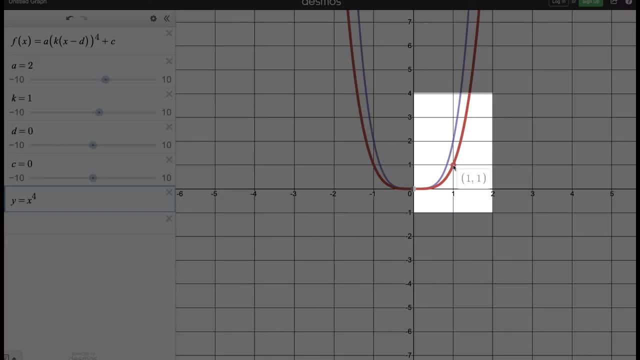 it looks like it's getting thinner and we call that it's being vertically stretched by a factor of 2.. All of the y-values are now twice as high. Just look at when x is 1.. When x is 1, the parent function is at 1, but the transformed 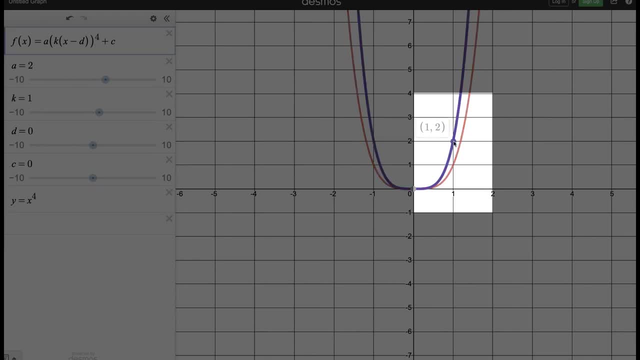 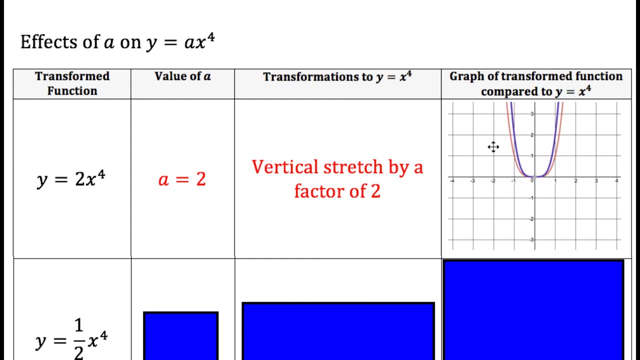 function will be twice as high. It'll be at 2.. So we say vertically stretched by a factor of 2, and draw the corresponding graph that's been vertically stretched For each x-value, the y-values are twice as high. If I make a a half, well, that would 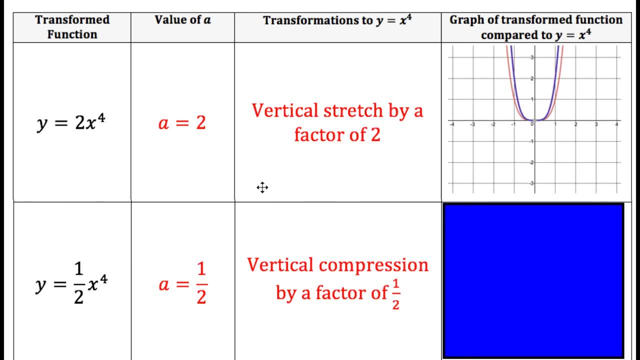 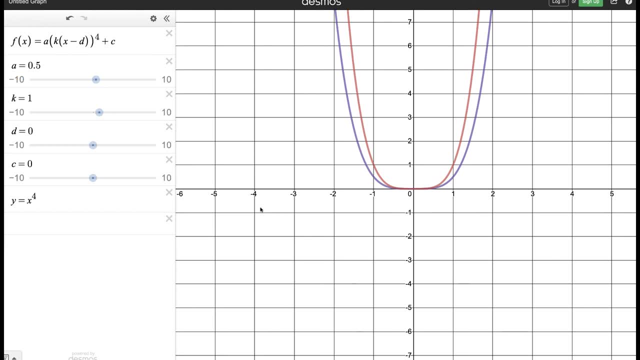 mean the y-values are going to be half as high. So that's a vertical compression by a factor of a half. So let me show you on here. Let's set a to a half and there we go. Notice that it's been vertically compressed. It's like someone from the top has squished. 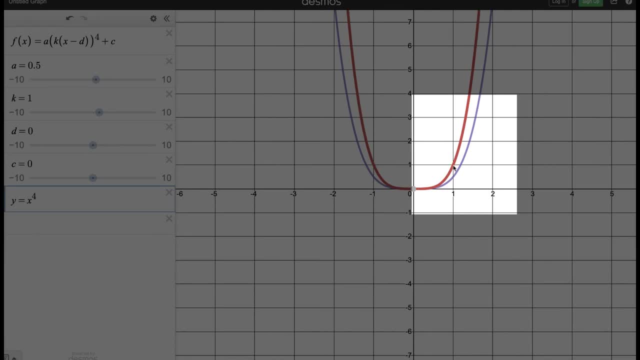 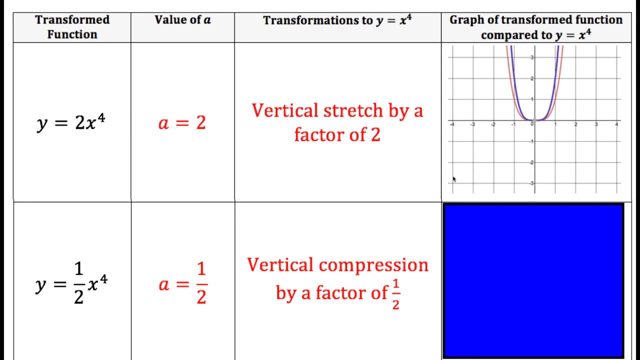 it down. When x is 1, the parent function is at 1, but the transformed function is half as high, It's at 0.5.. Let's make a negative. So when a is negative, 2, it's going to be. 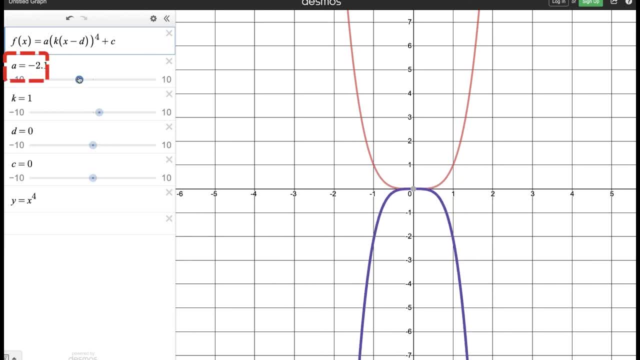 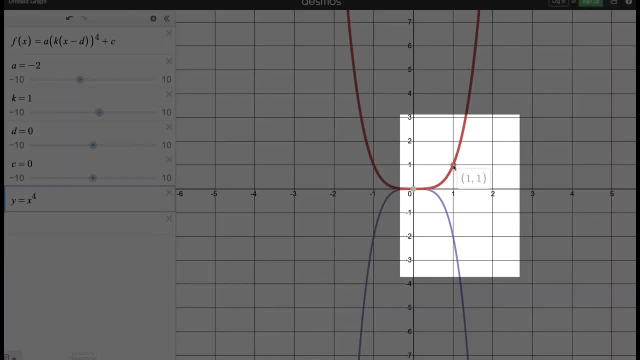 at 0.5.. Notice, it has also been flipped upside down. The original function, when x is 1, the y-value is at 1, but the transformed function, when x is 1, it's been flipped upside down and doubled, So it's down here at negative 2.. So we'd say two things for this a-value. 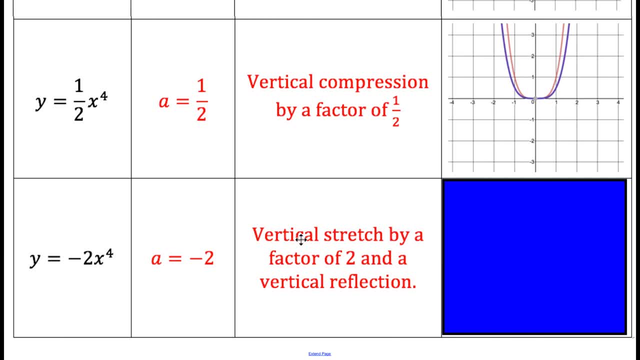 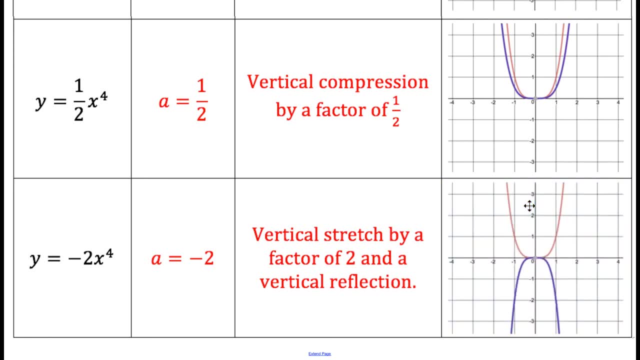 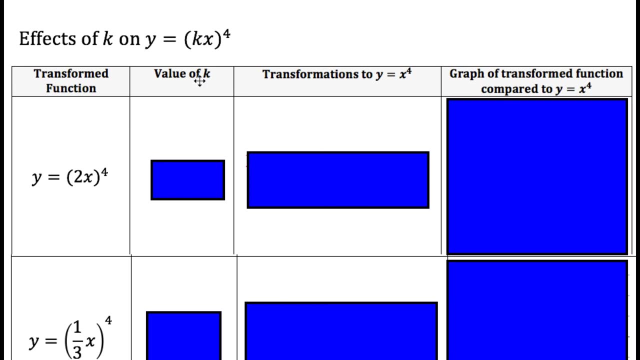 of negative 2.. There's been a vertical reflection and a vertical stretch by a factor of the absolute value of a. Let's look at k. k is part of the base of the power. That's how we can distinguish it from a, which was not part of the base of the power. So in this case the k-value is 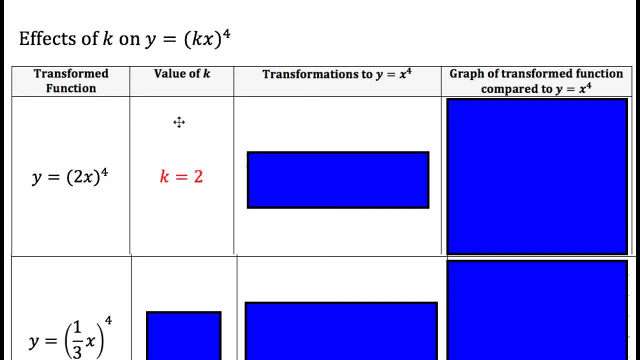 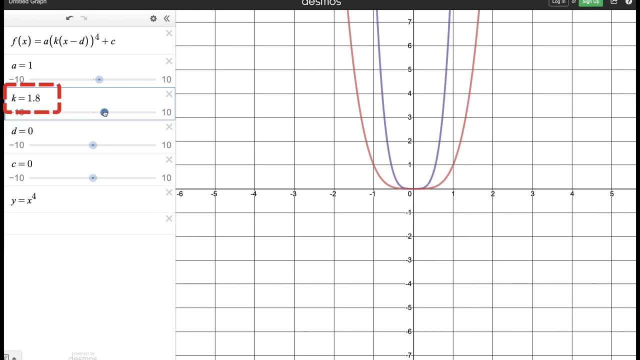 2. It's being applied to the x before the power of 4.. Let's look at what that does. If I increase k up to a value of 2, what's happening is a horizontal compression by a factor of 1 over the absolute value of k. 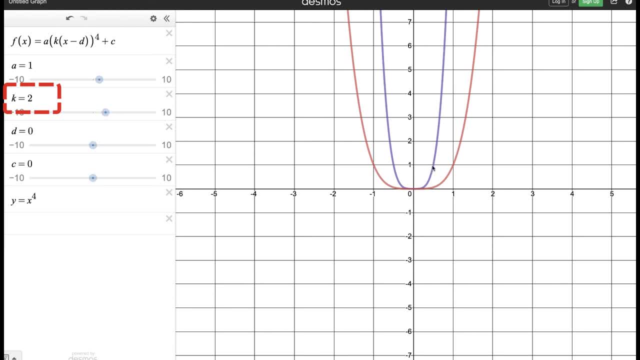 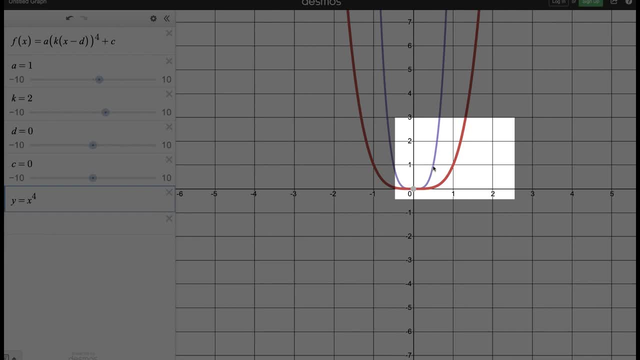 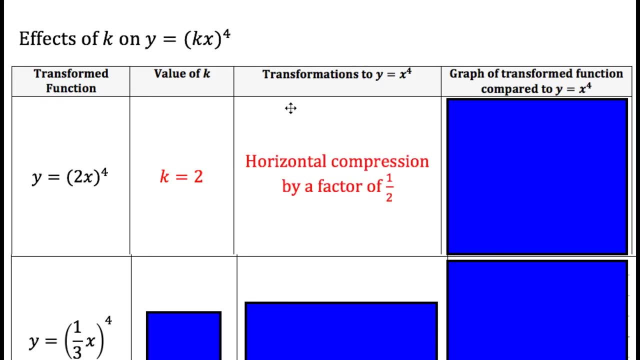 At any given y-value of the function, the x-value is now half as far from the x-axis. Here, at a y-value of 1, x is 1, but if I go over to here the transformed function, when y is 1,, the x-value is now half of that, It's 0.5.. So we'd say a horizontal compression. 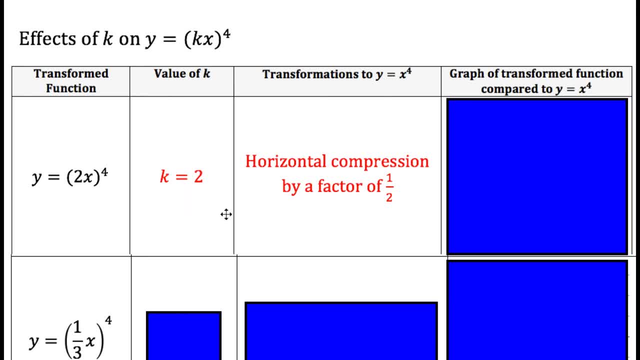 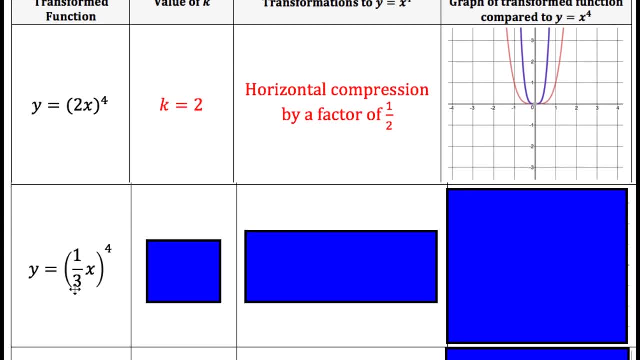 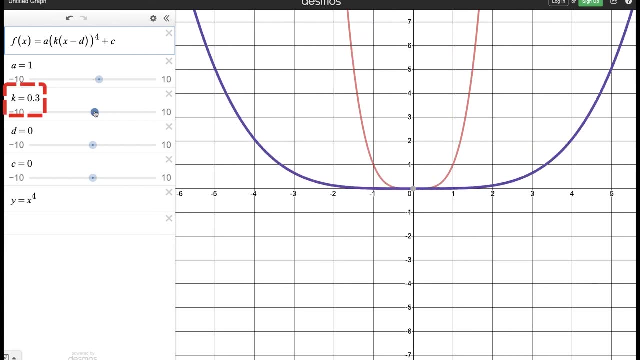 by a factor of 1 over the absolute value of k, And there's what the graph looks like: a horizontal compression. How about k? if k is a third, Let's set k to a third. Let me get it exactly a third. Let me write the fraction. There we go. Notice it's been. 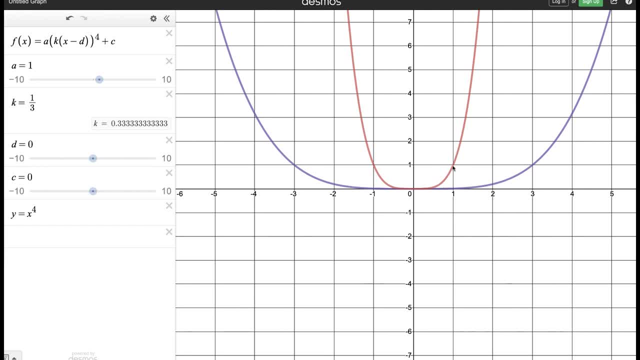 horizontally stretched. By what factor? Well, when the y-value was 1 on the parent function, we know x was 1.. When the y-value is 1 on the transformed function, what's the x-value? It's over. here It's been tripled, It's 3.. So it's actually been a horizontal stretch. 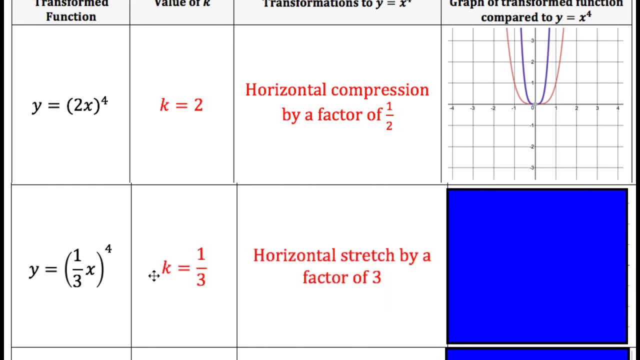 by a factor of 3 when the k-value is a third. So a horizontal stretch by a factor of 1 over the absolute value of k and 1 over a third. That means it's reciprocal. so 3. Here the k-value is negative. 2. For an even degree power function, that's actually going. 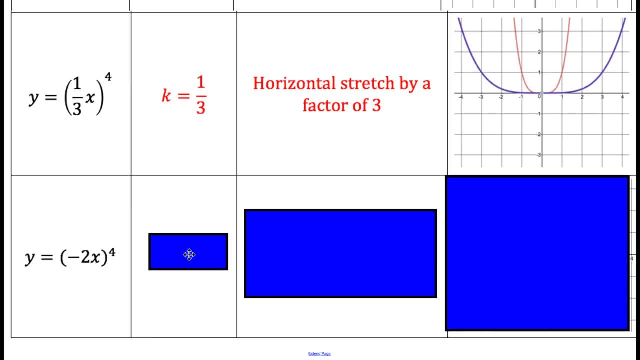 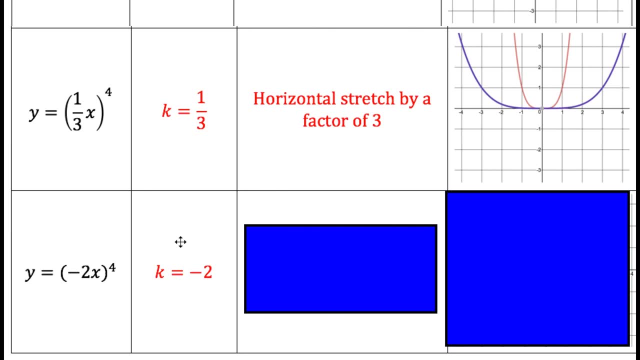 to do the exact same thing as a k-value of positive 2 did, because when k is negative it does a horizontal reflection. but even degree power functions are already symmetrical about the y-axis, so the horizontal reflection. you're not going to notice anything, Look. 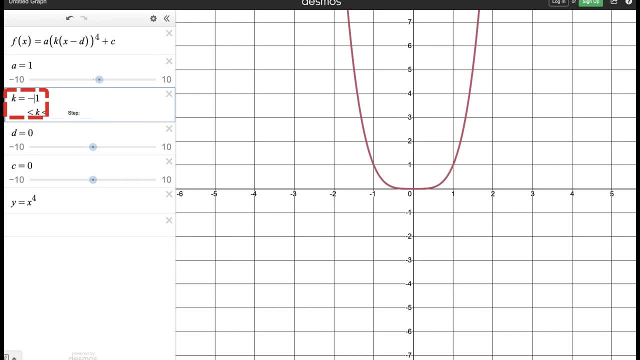 at what I mean If k is 1. Or negative 1. You don't see any change at all. Doesn't matter If it's an even degree power function. Odd, Different story. So let's set k to negative. 2. It's been horizontally compressed by a factor of 1 over the absolute. 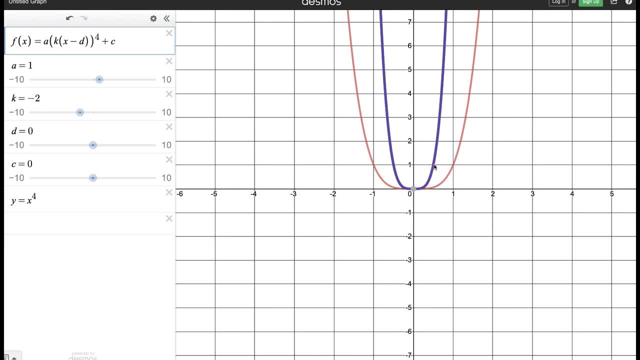 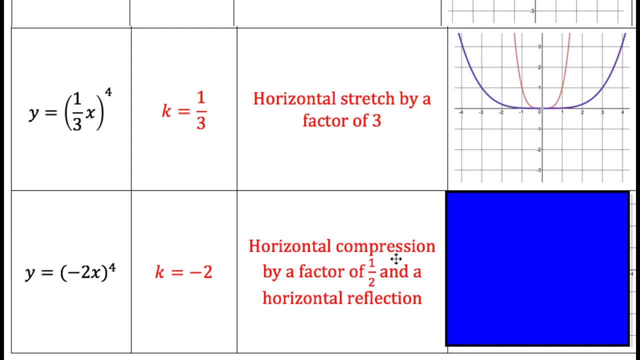 value of k, so 1 over 2.. So the x-values are half as far from the y-axis now, And there, technically, was a horizontal reflection, but it doesn't cause a change in the graph. And notice, when I'm describing the horizontal compression it's always by a factor of 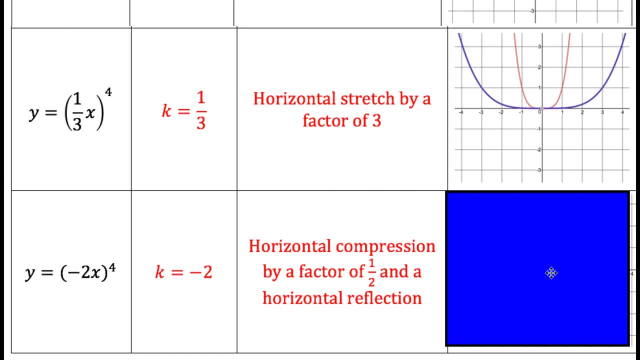 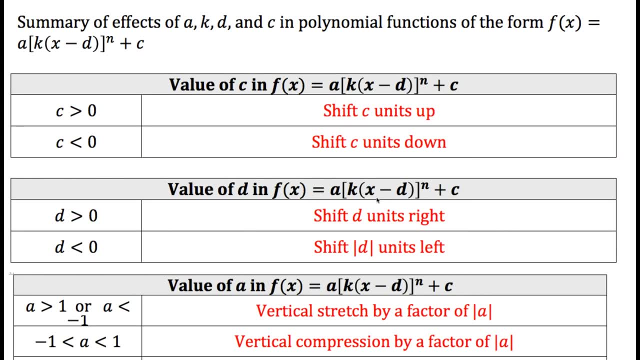 the absolute value of 1 over k. The negative is just what causes the reflection. Okay, so on this slide we have a summary of all the rules about what each parameter does and when it does it. So if c is positive, it shifts the graph up. If c is negative. 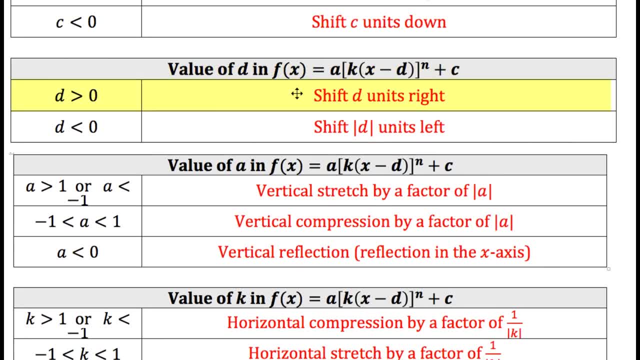 it shifts the graph down. If d is positive, it shifts right. If d is negative, it shifts it left. But keep in mind the d-value will always appear as the opposite sign of what it is, because of the fact that it's the general template for a transform. 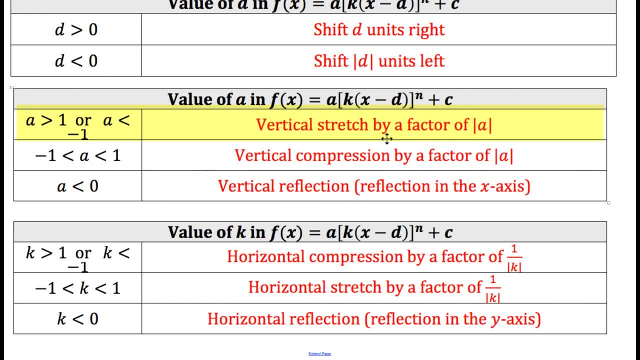 So the function is x minus d, a. does a vertical stretch by a factor of the absolute value of a, if a is bigger than 1 or less than negative 1.. Does a vertical compression by a factor of the absolute value of a is between negative 1 and 1.. 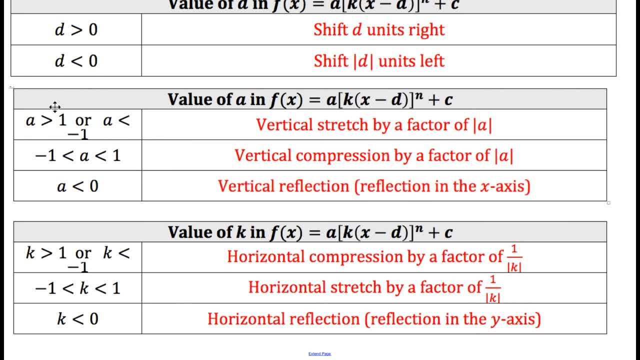 And if a is negative, we always say there's a vertical reflection. k is like the opposite of a. If k is bigger than 1 or less than negative 1, there is a horizontal compression by a factor of 1 over the absolute value of k. If k is between negative 1 and 1,. 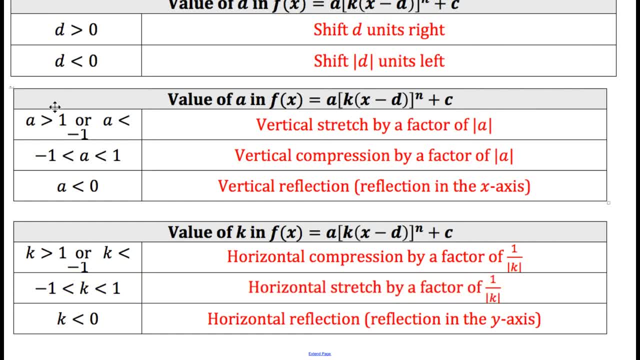 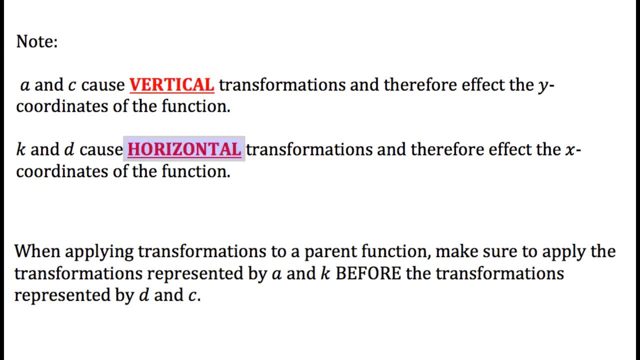 it's a horizontal stretch by a factor of 1 over the value of k and if k is negative there's a horizontal reflection, and i mentioned this already. but a and c cause vertical transformations and k and d cause horizontal transformations, which means algebraically, when we're coming up with transform, points a and c are going to affect. 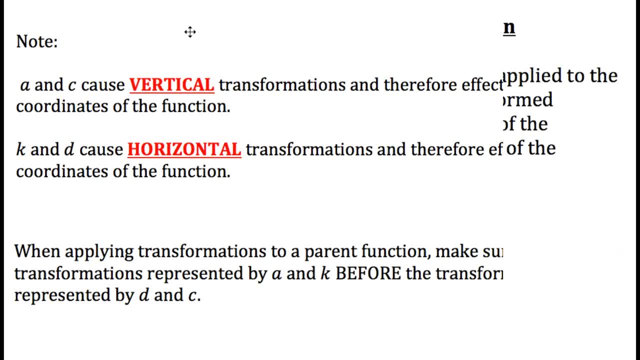 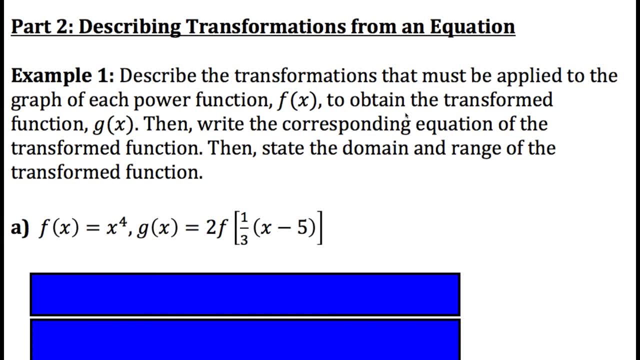 the y coordinates, k and d are going to affect the x coordinates. okay, let's complete part two, where we're going to describe transformations from an equation. so example one says: describe the transformations that must be applied to the graph of each power function, f at x to obtain the 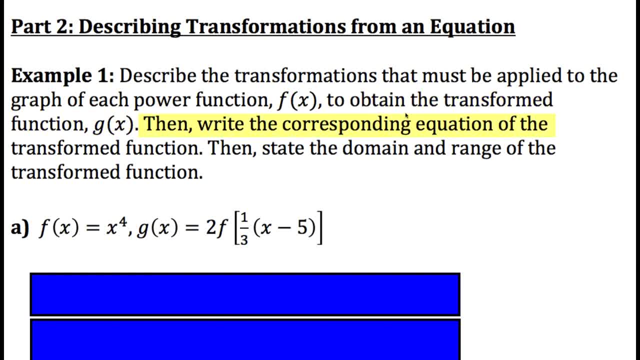 transformed function g at x, then write the corresponding equation of the transformed function, then state the domain and range of the transformed function. so in this question, part a, the parent function f at x is equal to the power function x to the fourth. and what's happening to? 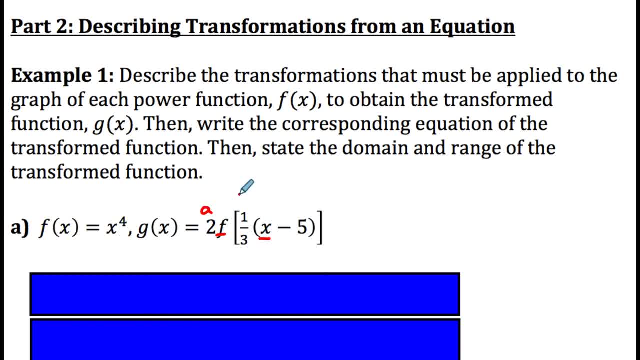 that parent function f at x is that an, a, k and d parameter are transforming it. well, it's actually stiff. start by writing the equation of the transformed function. Let's make sure we apply the horizontal transformations k and d to the base of the power right. It's f at this value. So what we have to do 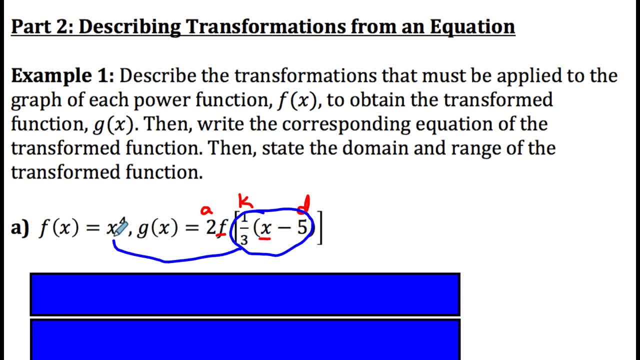 is in the f at x function. replace the x with that, So the transformed function is now a one third times x minus five to the power of four, instead of just an x to the four. And don't forget the a value goes out front of the power, so a two goes there. So that's the equation of the. 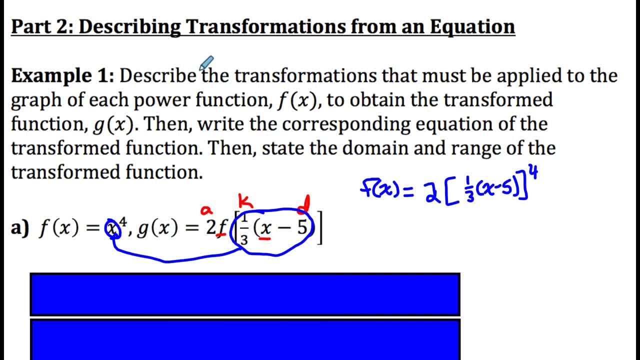 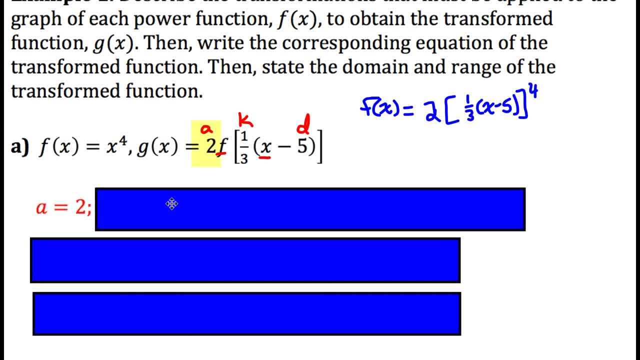 transformed function, knowing that the parent function is an x to the four function. Now let's describe what those parameters a, k and d are going to do to transform the function. Well, the a value we can see is two, That's an, a value bigger than one. so it's going to do a vertical stretch by a. 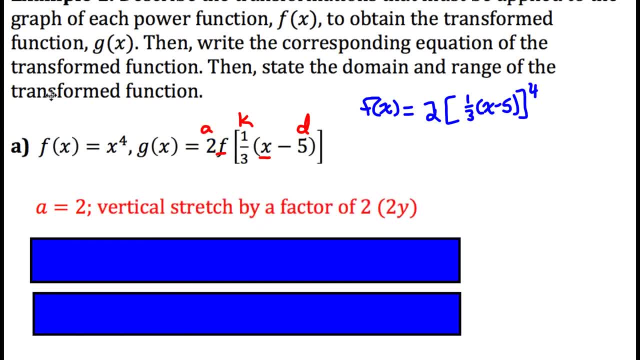 factor of two. So how we would apply that algebraically is we would double the y values. So in brackets you'll just see the algebraic transformation. for if we were to actually transform a table of values, which we'll do in the next example, The k value is a third. So this k value 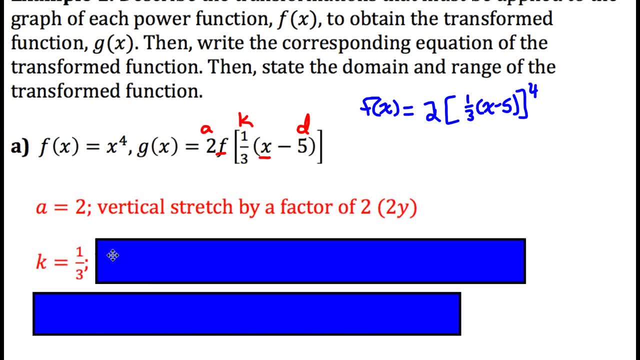 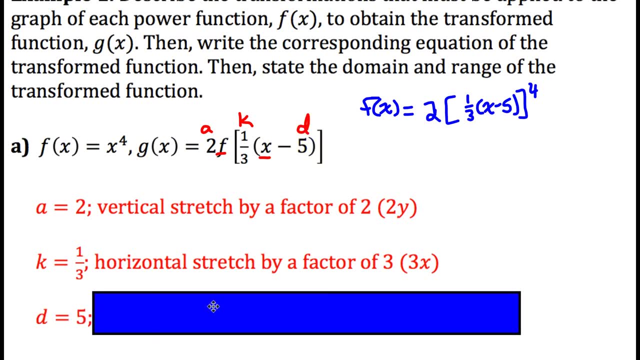 of a third, that's between negative one and one. so that does a horizontal stretch by a factor of one over the absolute value of k, so by a factor of three. So what that does is it triples all the x values And the d value is positive five. And what that does is it's going to shift the function. 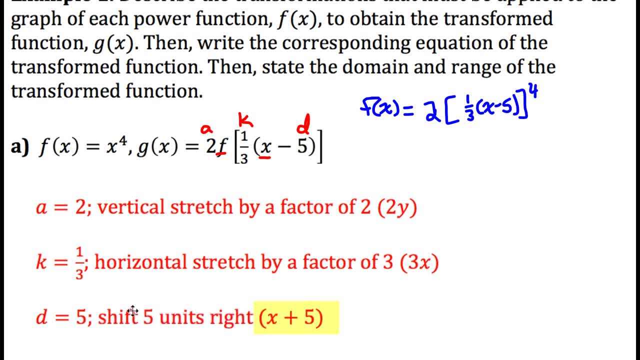 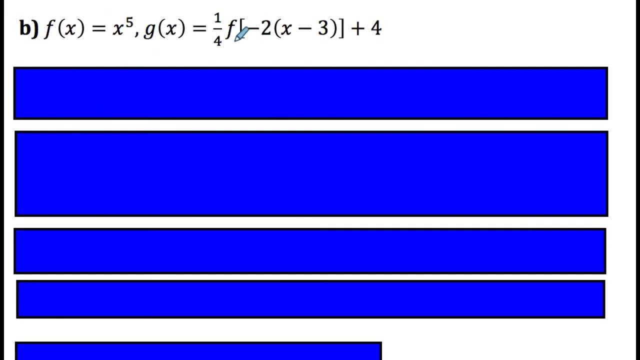 right five, and we could accomplish that by adding five to all the x coordinates. Part b: the parent function is now x to the five And our transform g at x is a transformed version of f at x. It has an a, k, d and c parameter, transforming it this time. So once again, 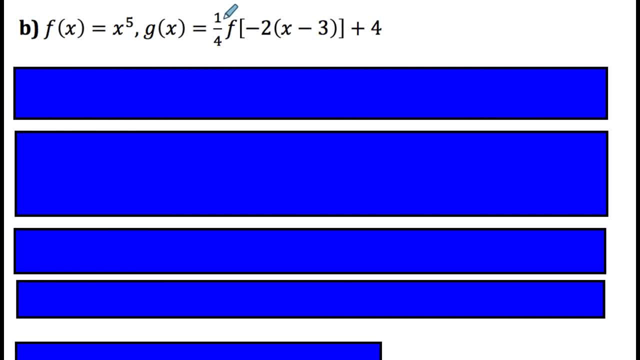 why don't we start by writing the transformed function's equation? So the transformed function g at x is the f at x function, but it's f at this. So we replace the x in the parent function with that, And then we'll apply the a and the c parameters outside of the 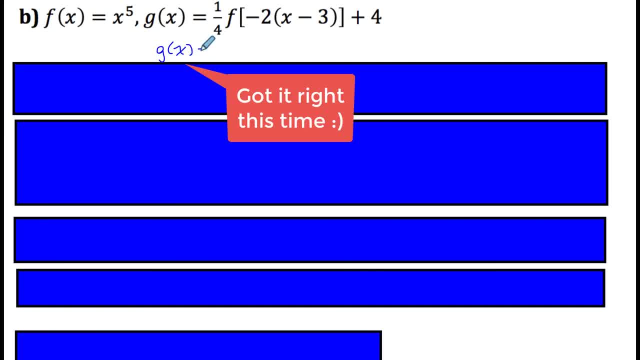 power. So the g at x function would equal this negative two times x minus three, being raised to the power of four, with the a value of a quarter and the c value of four being multiplied outside and added to that power. So now let's talk about what the a, k, d and c parameters do. 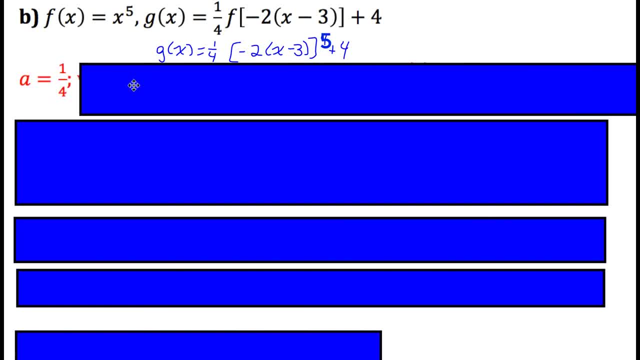 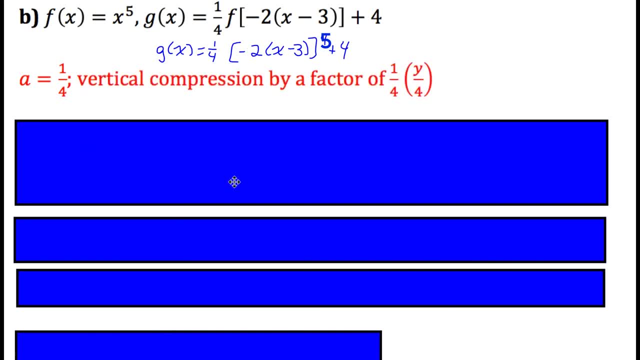 So the a value of a quarter, that's going to be a vertical compression by a factor of a quarter, because it's an a value between negative one and one. So what happens is the y values need to be multiplied by a quarter or divided by four, the k value of negative two, since it's less than. 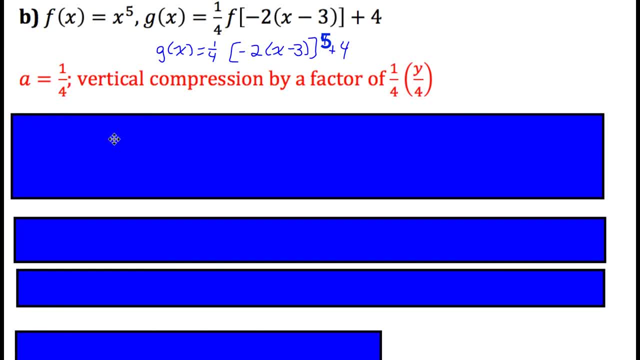 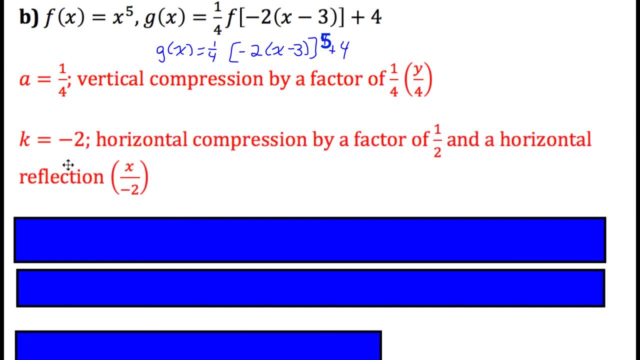 negative. one is going to do a horizontal compression by a factor of one over the absolute value of k, So by a factor of one over two, and then the negative is: what does a horizontal reflection? So what happens is we have to multiply the x's by negative half, or 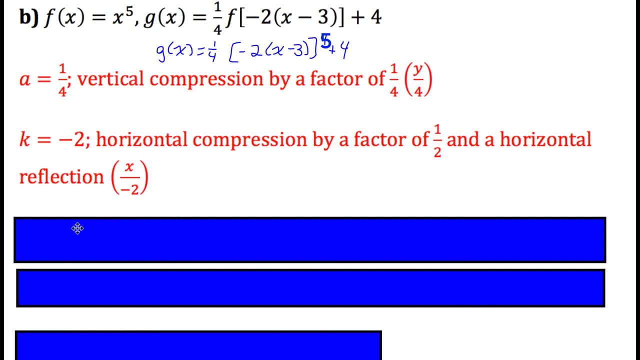 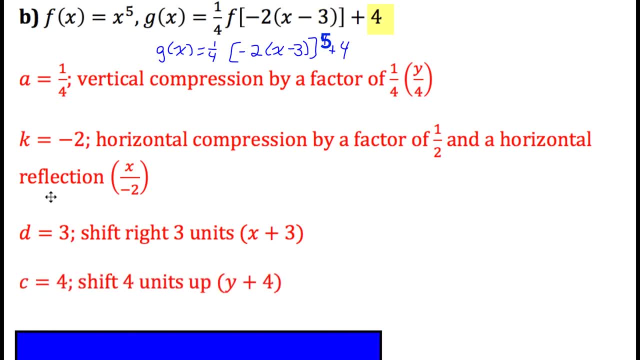 divide them by negative, two. same thing. The d value is three. that's going to shift it right three, so we'd add three to the x's, and the c value is four. that means shift it up four, which means add four to the y's. Okay, the next two examples are actually going to be graphing. 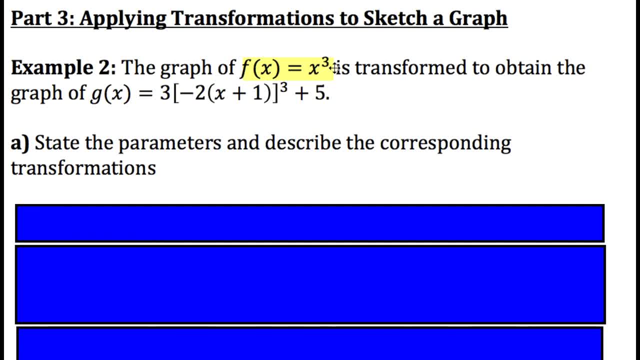 questions. Example two: the graph of x cubed is transformed to obtain this transformed function g at x, which has an a, k, d and c parameter doing the transformation. So before I actually graph this transformed function, let's state the transformations in. 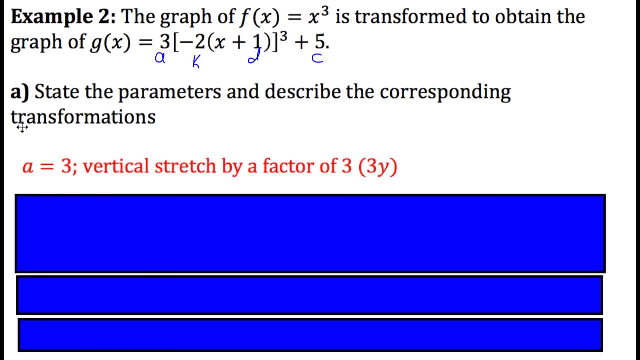 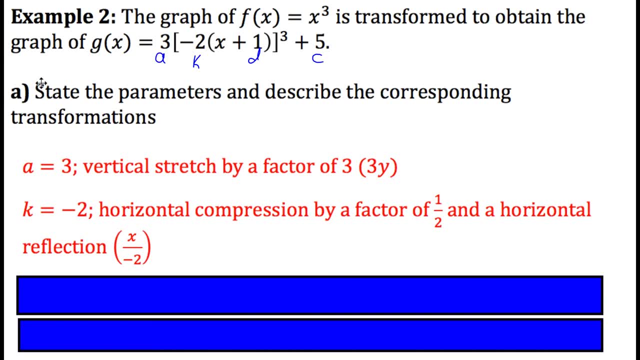 words again. So the a value is three, which does a vertical stretch by a factor of three. The k value is negative. two, which does a horizontal compression by a factor of one over the absolute value of k. so one over two, And the fact that it's negative means a horizontal. 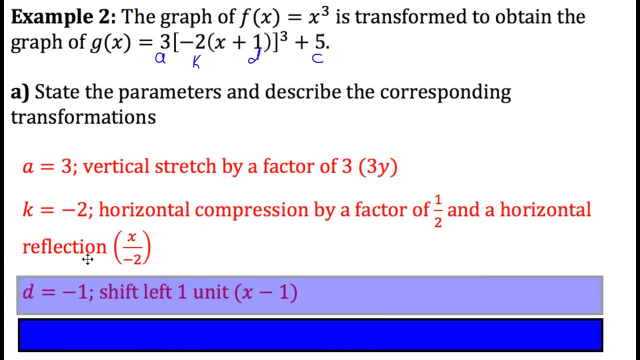 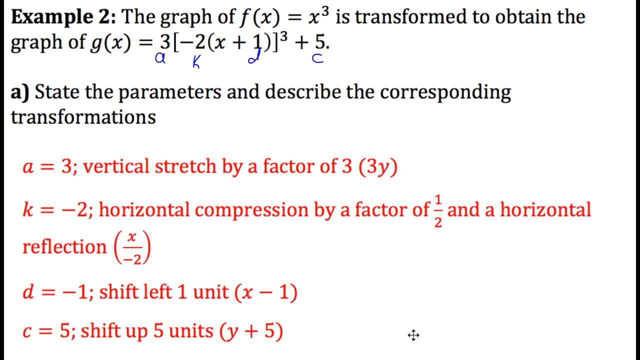 reflection D is negative, one which shifts it left one, and c is five, which shifts it up five. And notice brackets. I have all the algebraic transformations which accomplish what I've written in words, which is what we're going to have to do- to a table of values of points, to come up with points for a. 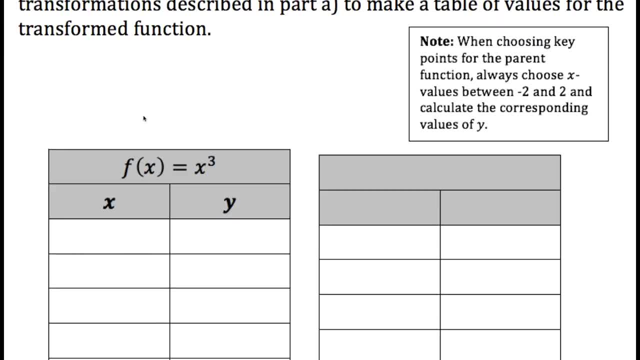 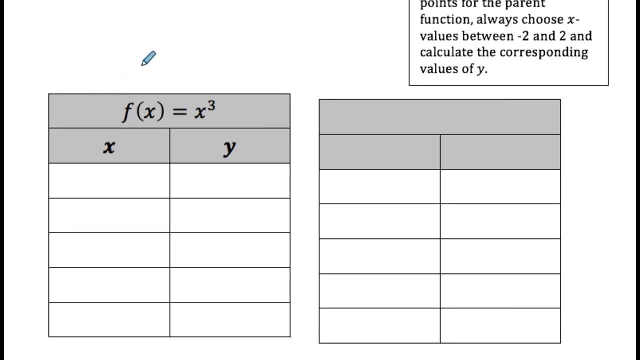 transformed function. So when we do these questions, we're always going to fill out two tables. We're going to fill out a table of values for the parent function, x cubed, And for that parent function we're always going to choose x values, negative two, negative one, zero one. 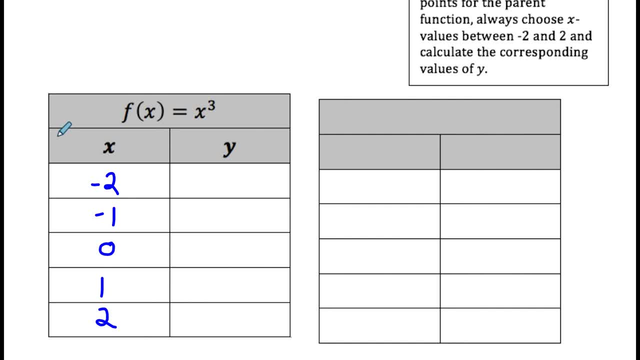 two. Those x values will give us a good shape of the parent function which will then result in a good shape for the transformed function. So if I plug these x values into this x cubed equation of the parent function, negative two cubed is negative eight- negative one cubed. 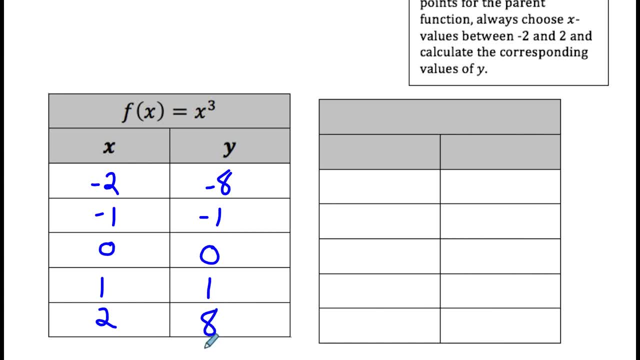 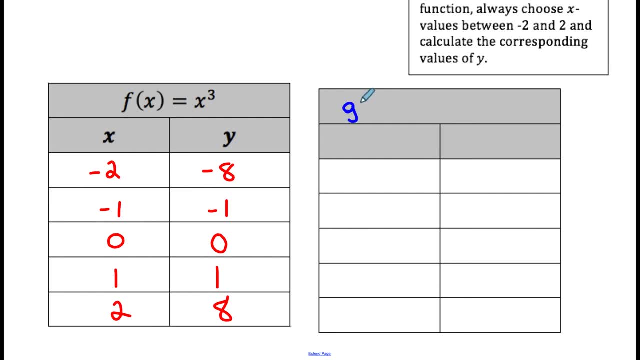 is negative. one zero cubed is zero. one cubed is one. two cubed is eight. These are points for the parent function. Now let me do the table of transformed points. So this table is going to be for our g at x transformed function. Okay, so let's figure out what's going to happen. 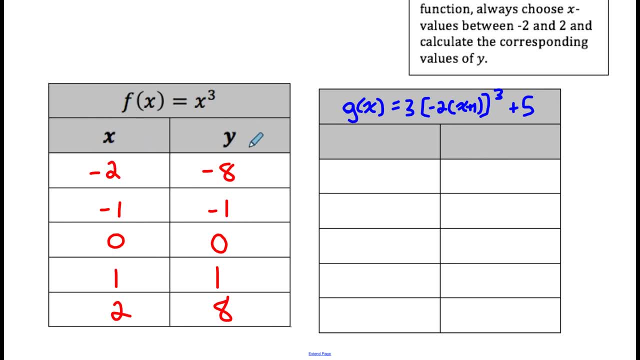 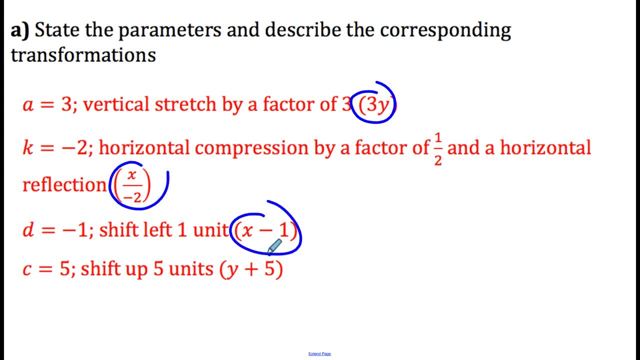 transformation-wise to the x values and the y values, The general template of what we do transformation-wise. I mean, we already wrote them over here that we're going to do so. we just have to apply those transformations to our table of points for the parent function and then we get a table of points for the transformed function. 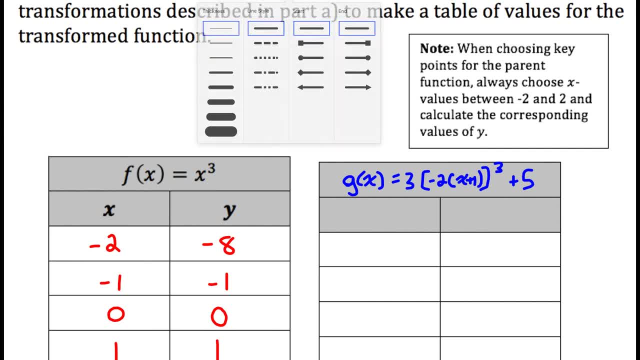 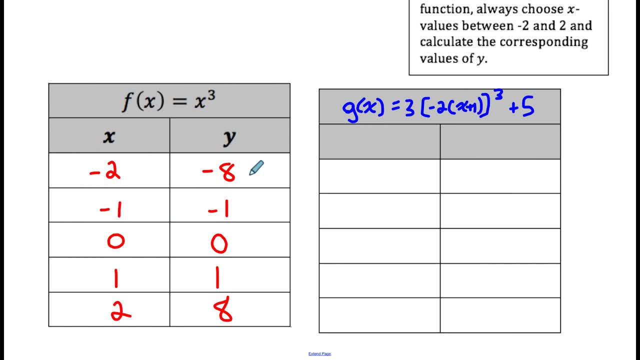 The general template that you can follow would be to get the transformed values for x. we take these x values and do each of those x values divided by k, because the effect of k is always done by its reciprocal. So we do x divided by k and then we have to do the horizontal shift by adding the d value. 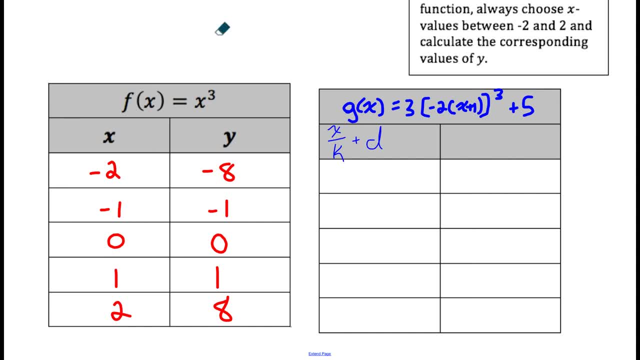 So you can always do x over k plus d. So in this case that would mean: to each of the x values we divide them by negative two and then add negative one, so I could just write minus one. And to the y values what we always do is we multiply the y values by 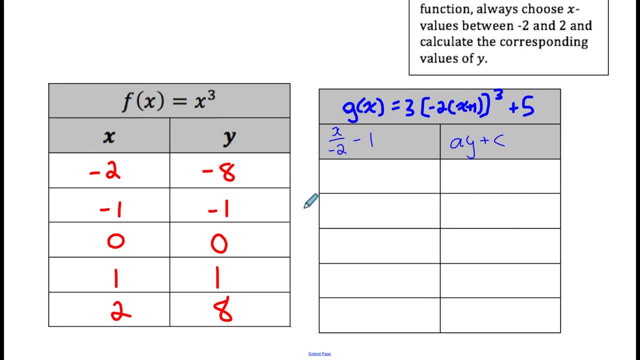 to do the vertical stretch or compression, and then we add the c value to shift it up or down. So ay plus c is what we always do there. So in this case it would be 3y plus 5.. So we need to do those sets of transformations to these x and y values and then we get points. 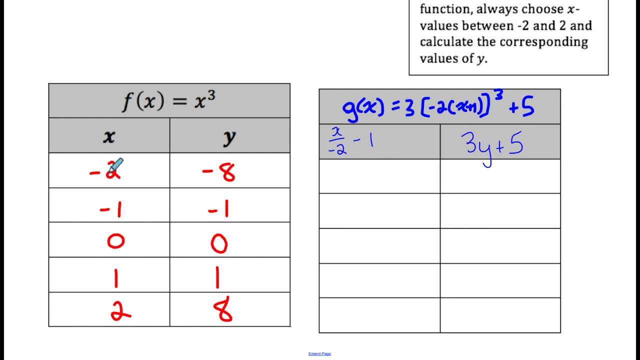 that are on the transformed function. So let's take all of our x values and plug them into here for x, and then we will get the x values for our transformed function. So let's start with negative two, So we plug it in for x into there. We would get negative two over negative two, which is one. 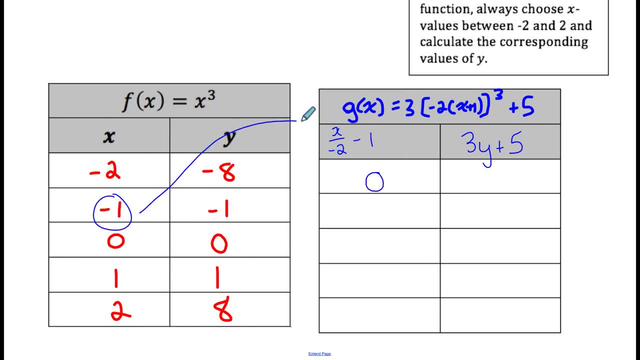 minus one is zero. Now let's take negative one. plug it in for x and we would get a half minus one, that's negative a half. Plug zero in, we would get negative one. plug one in, we get negative 1.5,. plug two in, we would get negative two. So those are the x values for the transformed function. 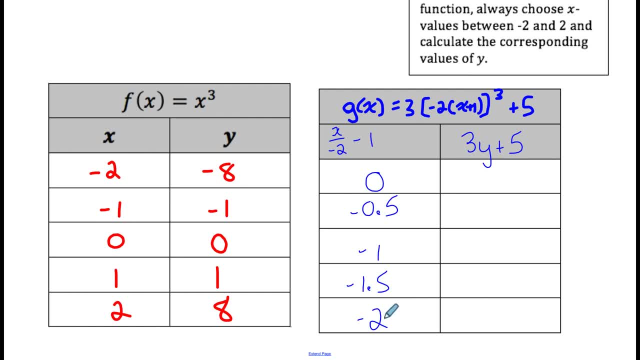 now to get the y values. I guess we have a couple of options. What I'm going to do is do these transformations to these y values, but I suppose what I could do is I could take these x values and plug them into x, into the transformed equation. We should get the same answer either way. 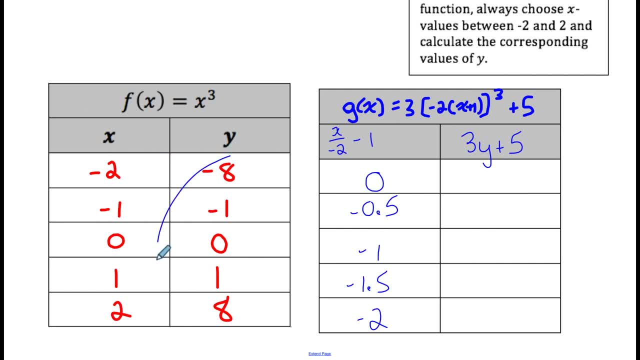 and it would be a good way to check your work. But let me transform these y values. that's the way I'm going to do it. So I'm going to take negative eight and plug it in for this y value, So it'd be negative 24 plus five. that's negative 19.. 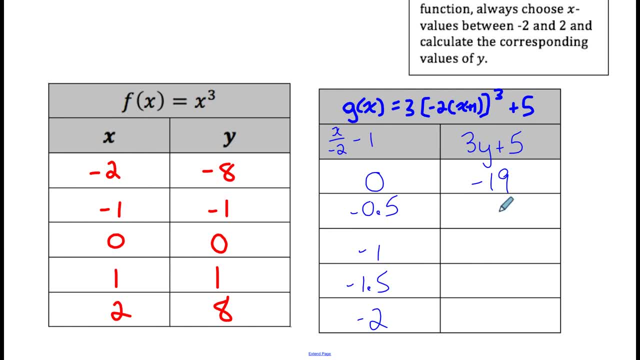 Take negative one, plug it in for this y value Negative. three plus five is two. plug zero in, get five. plug one in, get eight plus eight in, I get 29.. So here's a table of points for the transformed function. Let's graph the parent function and. 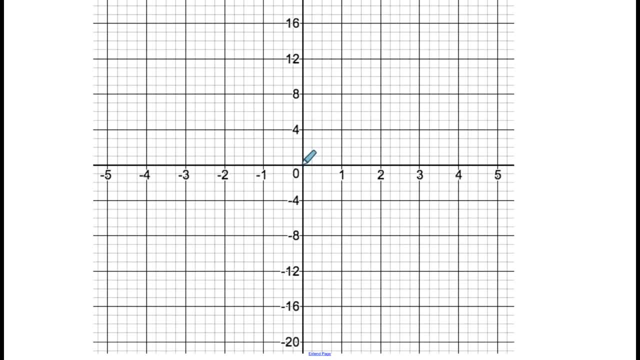 the transformed function. So parent function: zero, zero, one, one, two, eight. negative one negative, one negative, two negative, eight. Just careful with the scale here. So there's my f at x function, and now we'll do the transformed function. 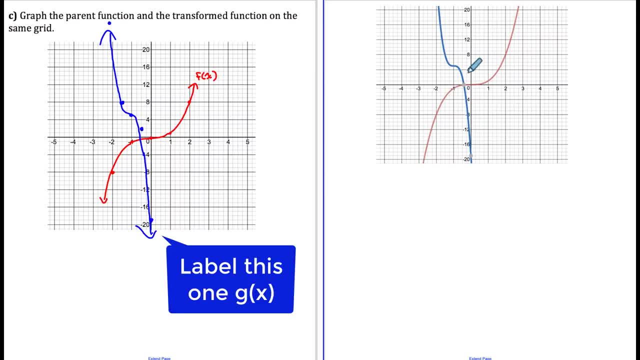 Okay, there's a rough sketch of the graph and we can compare that to what Desmos would give us. It's pretty accurate. Now you should always do a check after What you wrote in words about the transformations should match what it looks like on your graph as well. 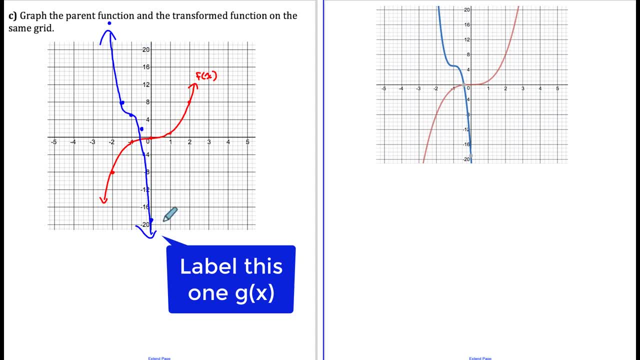 In words, we said it was going to be vertically stretched and horizontally compressed, so it should be a lot thinner, which it is, And we said it was going to move left and up, which it did. Good, Let's do one more practice of the same type of question. 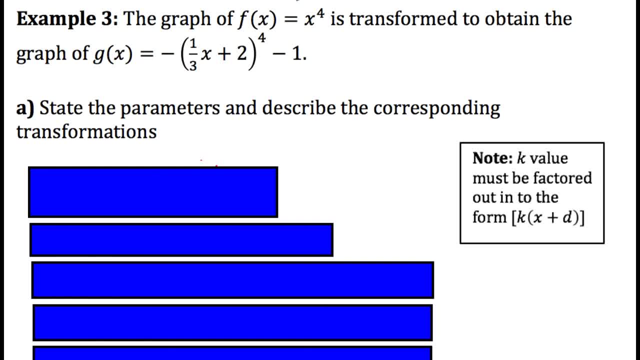 This time the graph of x to the four is being transformed, and here's the transformed version of it. But remember, the transformed version of a function should always have the k value factored out from x plus d in the base of the power, And this one doesn't. This one-third is: 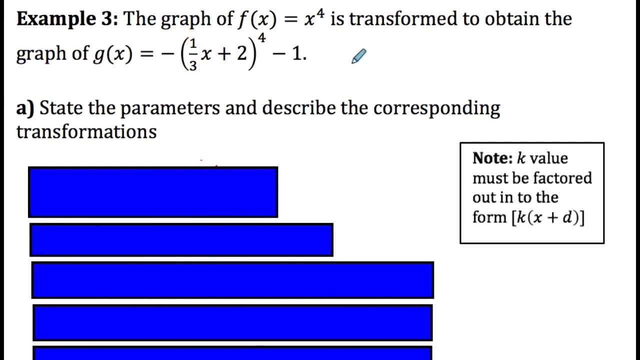 not a factor of x plus two. So what we need to do is factor out that one-third to get it into this format for the base of the power. So if I start by doing that, divide the third out from the x and the two, that leaves me with x and six, A third. x divided by a third is x and two divided. 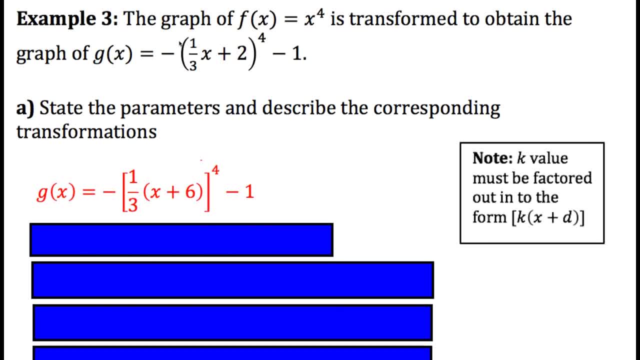 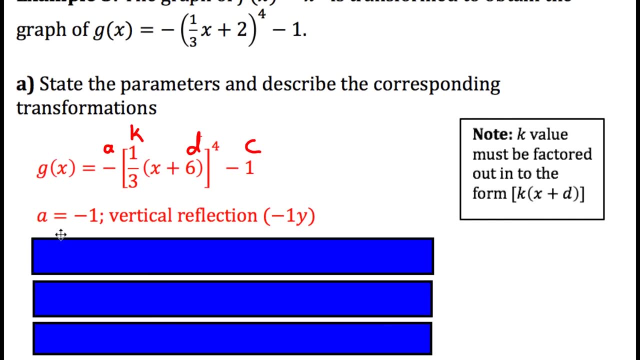 by a third is six. So now that it's in the proper format, you should be able to tell what your a, k, d and c values are. The a value is negative one, which is going to cause a vertical reflection, No stretch or compression, because multiplying things by one doesn't make them bigger or smaller. 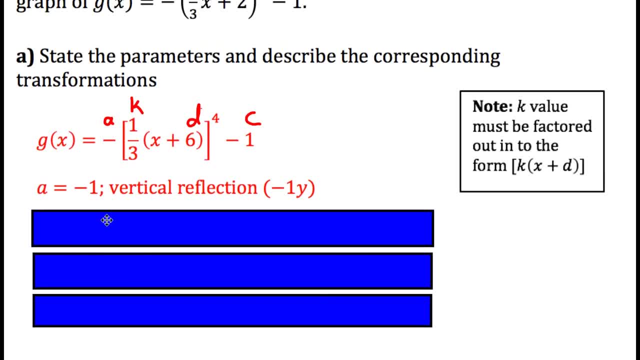 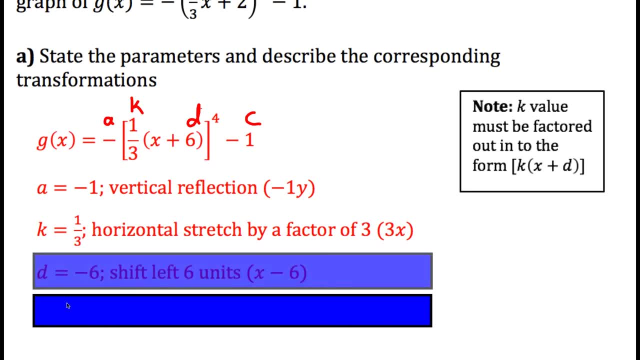 the negative just does the vertical reflection. The k value is a third, so that's a horizontal stretch by a factor of one over a third, which is three. The d value is negative six, which means move left six, and the c value is negative one, which means move down one. 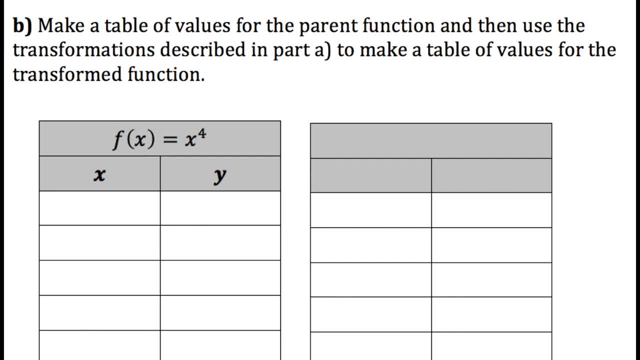 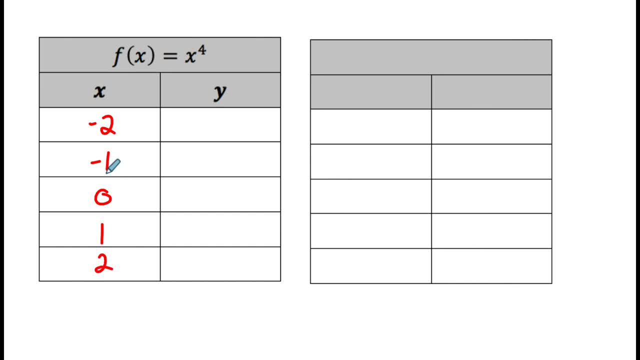 So let's do those transformations to the x, to the four function. So we need some key points for that parent function. so choose the same x values negative two, negative one, zero one, two. Plug them into this function to get the y values Negative two to the four is: 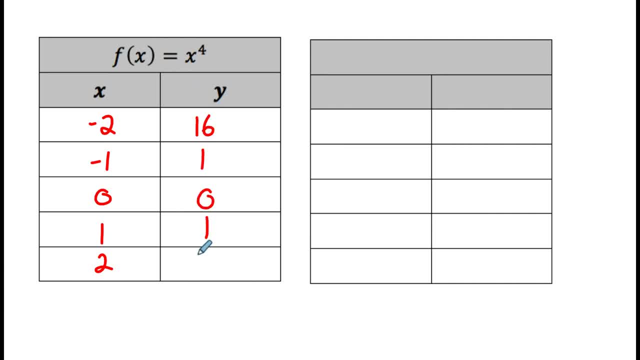 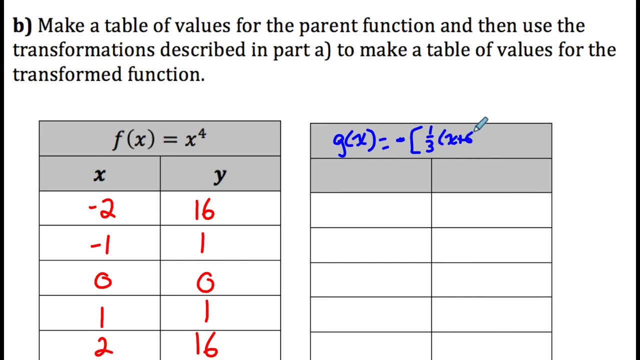 sixteen. negative one to the four is one, and so on. And now we're going to transform those points to come up with the equation for our transformed function- and it was g at x equals negative a third x plus six to the power of four minus one. So if we follow the general template we're supposed to follow for 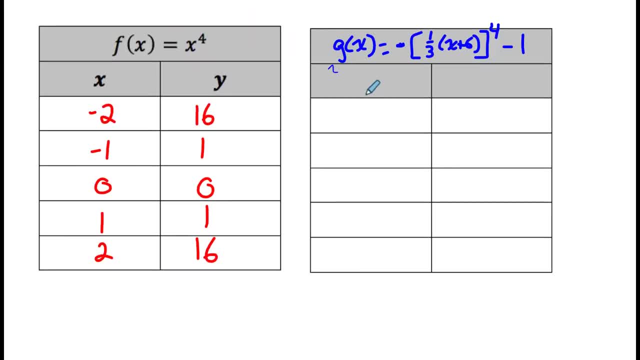 transformations. and if we just follow what we wrote in words, we do x over k plus d here and a y plus c here. So when I do x over k, x over a third, well that's just three x and plus the d value of negative six. so that would make this minus six. 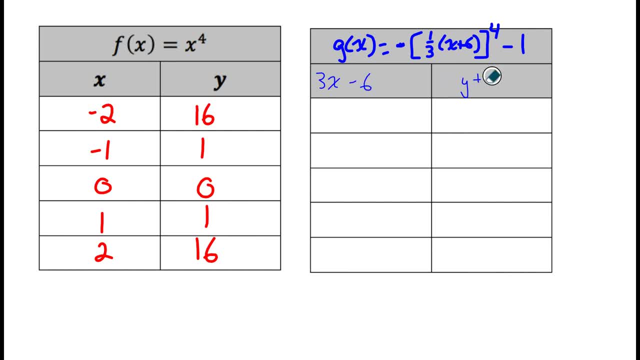 And a, y plus c. well, a is negative one and c is also negative one. so it's negative y minus one. This will perform the correct transformations to these points. So take each of the x values, plug them into three x minus six. take each of the y values, plug them into negative y minus one. 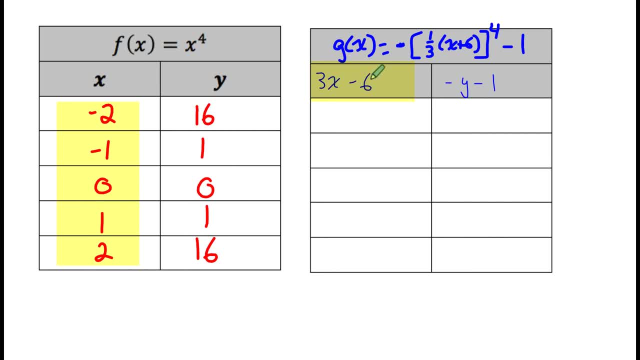 and let's see what we get: Three times negative, two is negative, three negative two is negative. two Negative six minus six is negative twelve. plug in negative one, we get negative nine. plug in zero, we get negative six, and so on. Now the y values plug in sixteen. 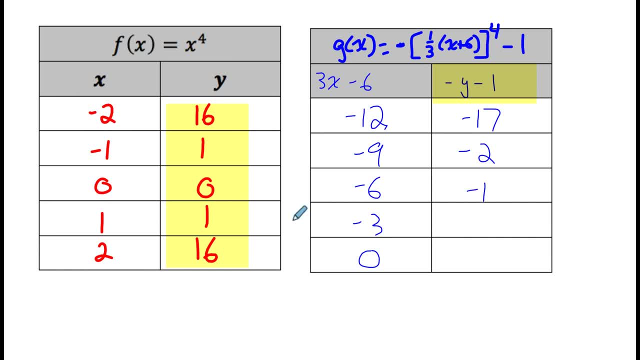 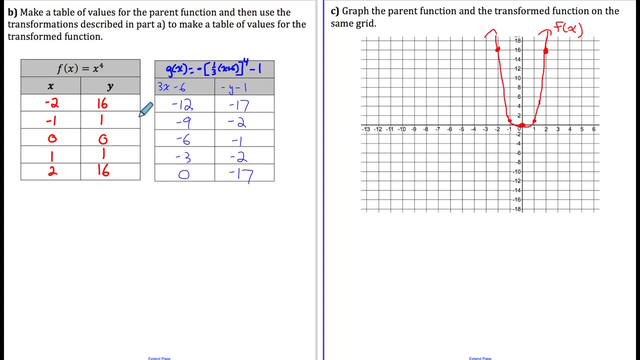 plug in one, plug in zero. plug in one again, plug in sixteen again. There's the table of points for our transformed function. Let's graph them both. There's the parent function and now let me do the transformed function. And there's the transformed function. Make sure you have both functions labeled. 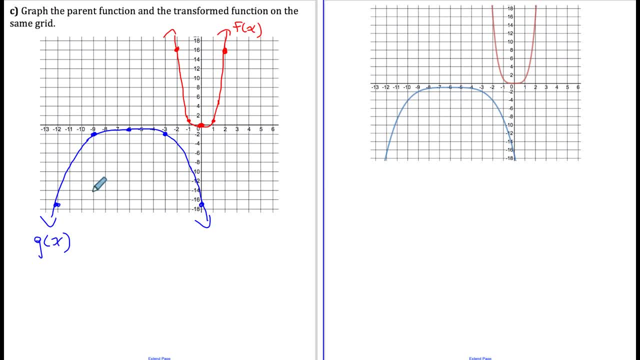 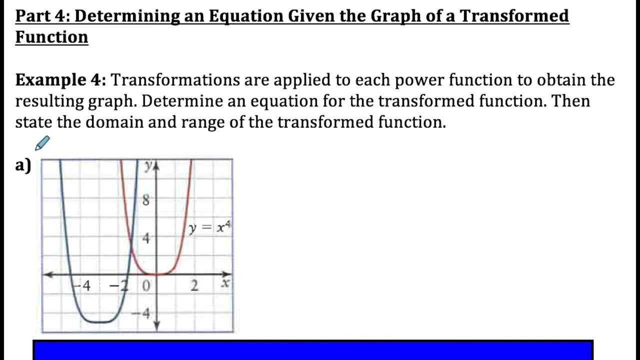 and let's compare it to Desmos, Looks like we have a good representation of the transformed function. Last part of this lesson: we're going to go backwards. I've given you the graph of a transformed function and we're going to write its equation. Example four says transformations are. 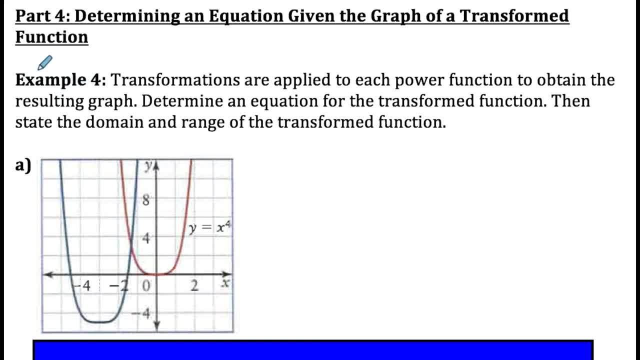 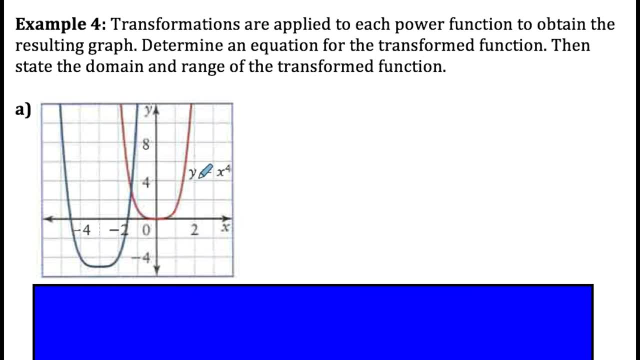 applied to each power function. to obtain the resulting graph, Determine an equation for the transformed function. then state the domain and range of the transformed function. For this one, the red one's the parent function. x to the four, the blue one has been transformed. It looks like. 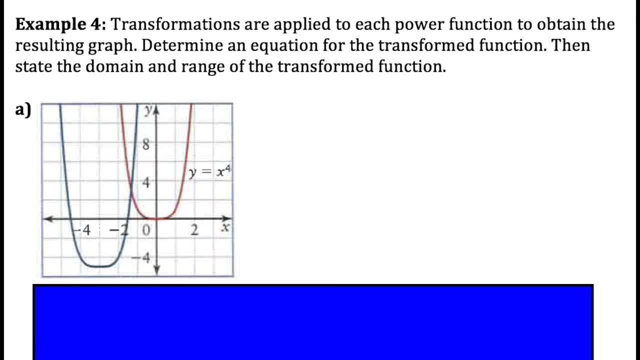 it's the exact same shape. it's just been shifted. To figure out the shift, let's compare the vertices. This vertices is at. this is at It looks like. We'll estimate that's what it is. So in order to get the to do that shift, we'd have to go left. 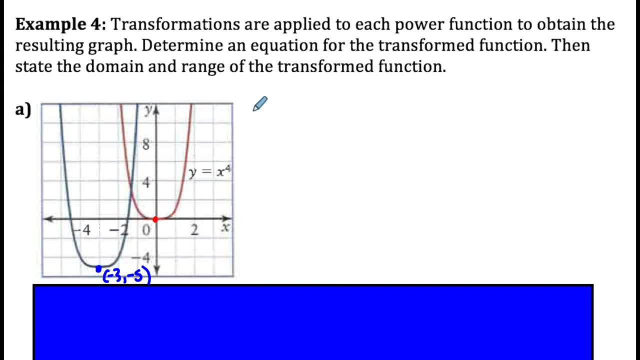 three down five. Left three down five. Well, to move left three, the d value would have to be negative three, and to move down five, the c value would have to be negative five. So our transformed function- I'll call it g at x, you can call it whatever you want- equals the x to the four. 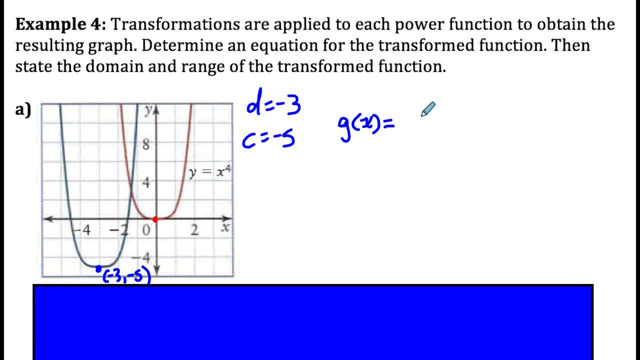 function with those two parameters applied. So the d value is going to be applied to the base of the power, so it'd be x plus three to the power of four, and the c value is added after, so plus negative five. So that's our transformed function. It also asks us to write domain and range. 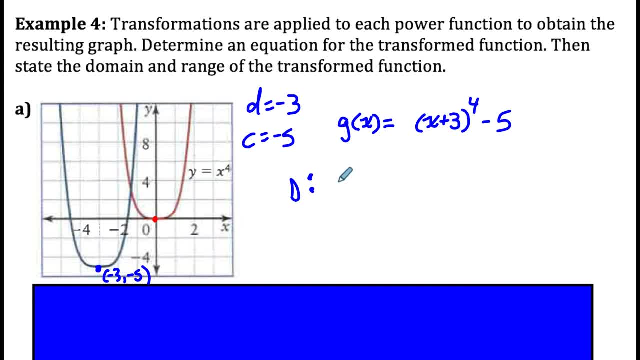 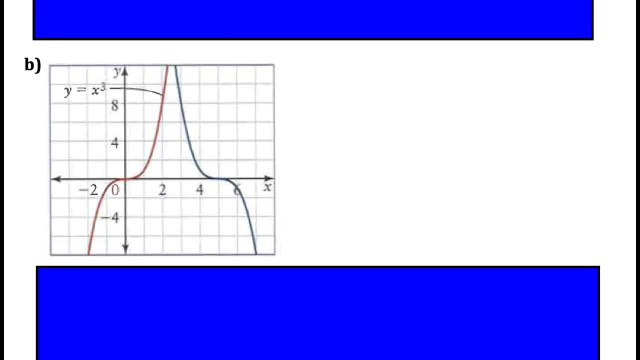 Domain. well, for power functions, the domain, there are never any restrictions, it's just from negative infinity to infinity. The range, however, for this one notice, it never goes below a y value of negative five. so we'd say from negative five to infinity. Part b. so the red one is the parent. 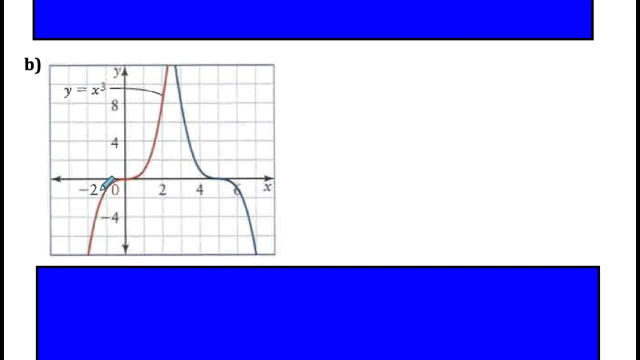 function x cubed. the blue one is the transformed function. If I look at this point right here, where is that moved to? It's been moved right five. so to go right five the d value would have to be five. But there's also been a reflection. that's happened and it. 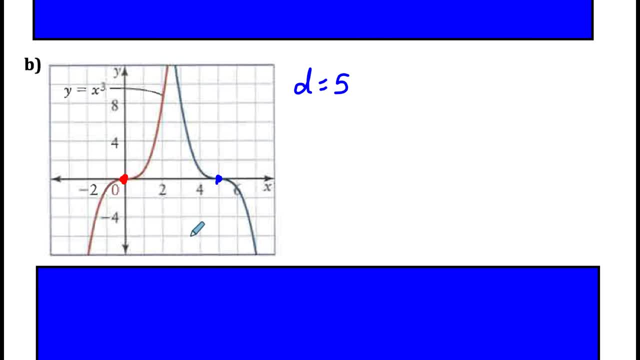 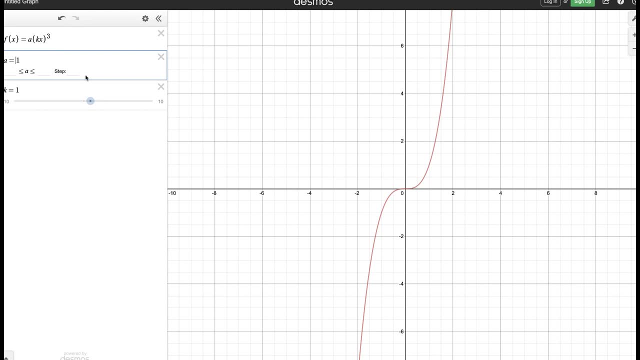 could be a vertical or a horizontal, They would actually do the same thing for this. so you can pick either one that you want. Let me just prove to you that they do the same thing in Desmos. Okay, so there's x cubed. It wouldn't matter whether I made a negative one. 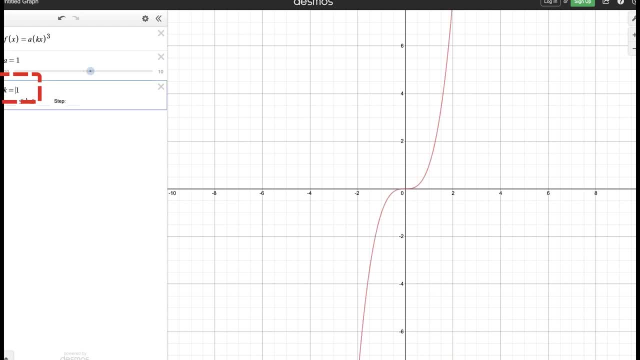 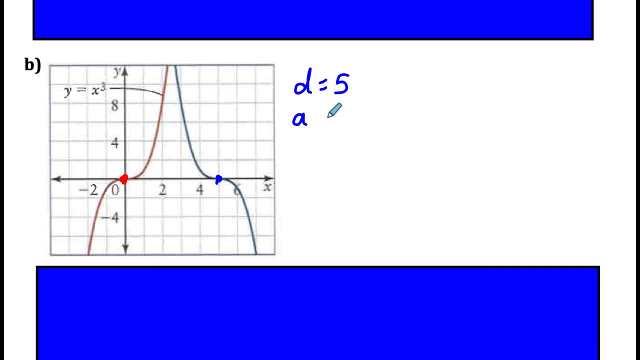 or k negative one. They would do the same thing, So we can choose whichever one we want. I will choose the a value to be negative one in this case. So my transformed function g at x would equal negative. the a value has to go outside the base. 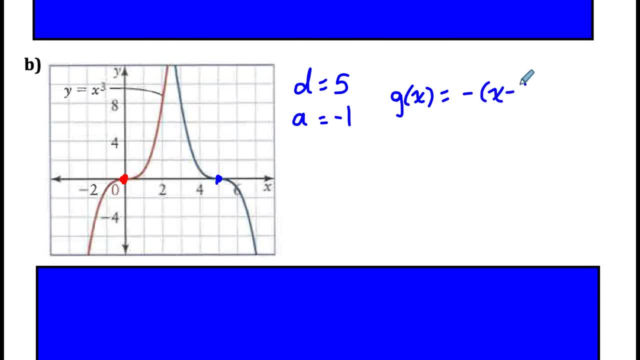 of the power, and the base of the power would be x minus five. Don't forget to cube it, because the parent function is x cubed. So there's my transformed function. It says domain and range For odd degree power functions. there's no restrictions on either, So for both of these we would just say negative. 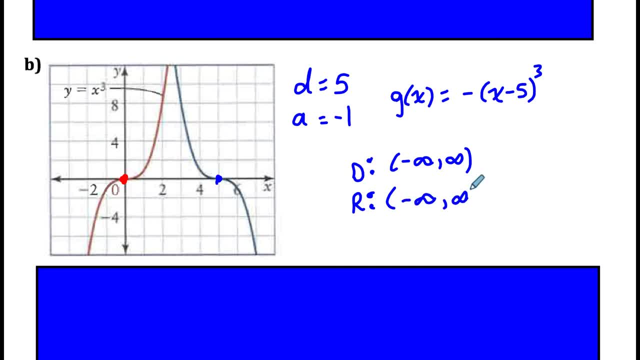 infinity to infinity. Okay, that's it for that lesson.